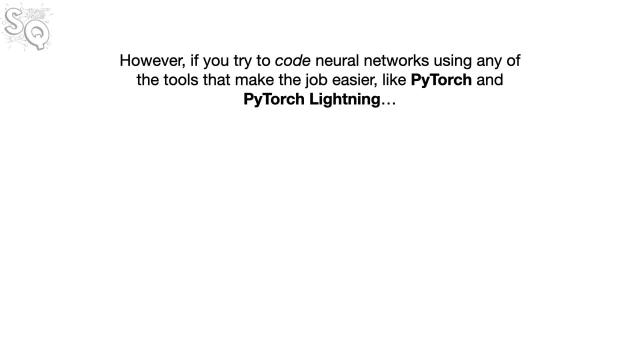 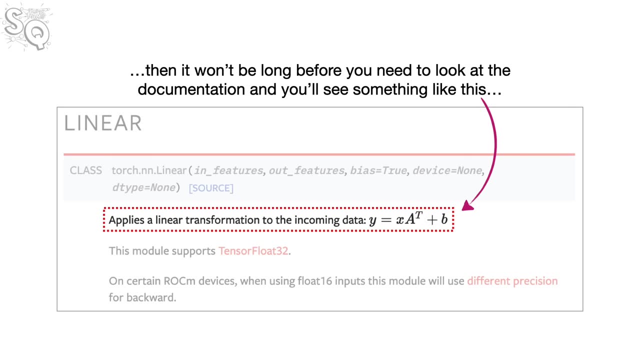 If you're using neural networks, using any of the tools that make the job easier, like PyTorch and PyTorch Lightning, then it won't be long before you need to look at the documentation and you'll see something like this: Ugg. Or you'll have a small bug in your code and you'll see an error. 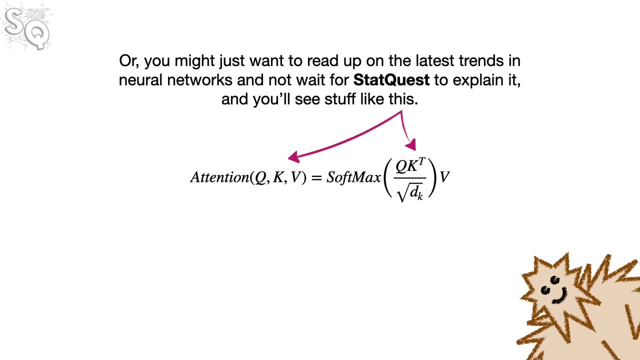 like this Double Ugg. Or you might just want to read up on the latest trends in neural networks and not wait for StatQuest to explain it, and you'll see stuff like this Triple Ugg. All this math looks complicated and hard to understand. Don't worry, Squatch, We're going. 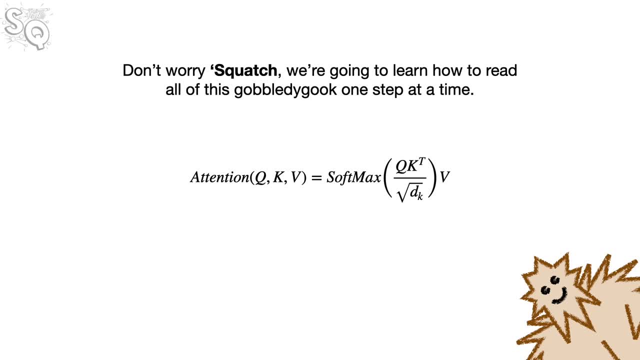 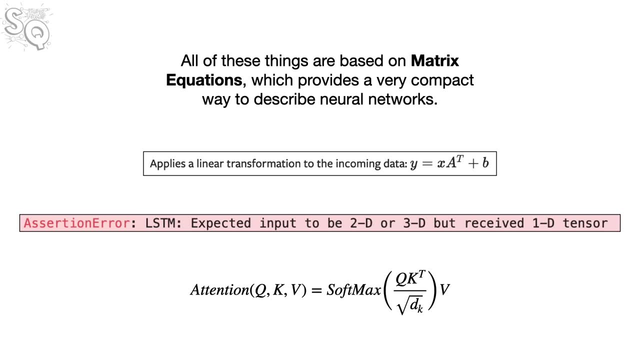 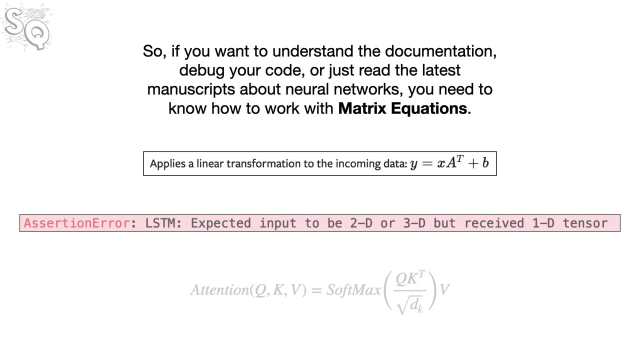 to learn how to read all of this gobbledygook one step at a time. Bam, All of these things are based on matrix equations, which provides a very compact way to describe neural networks. So if you want to understand the documentation, debug your code or just read the latest. 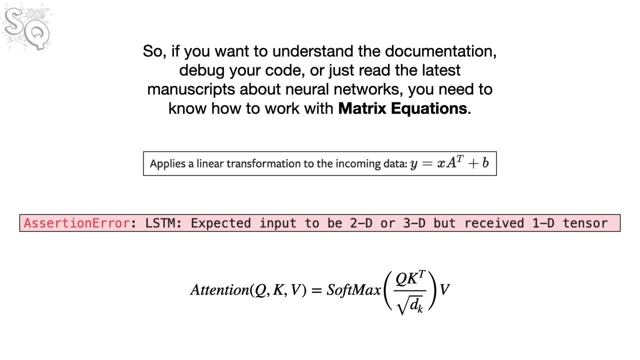 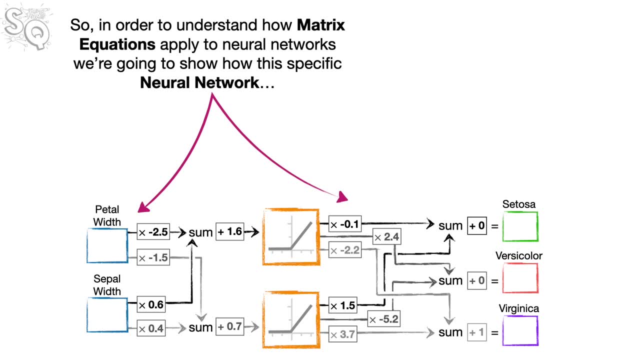 manuscripts about neural networks, you need to know how to work with the documentation. So, in order to understand how matrix equations apply to neural networks, we're going to show how this specific neural network translates into this compact matrix equation. Ugg, That equation looks weird. Are you sure I'm going to understand it? 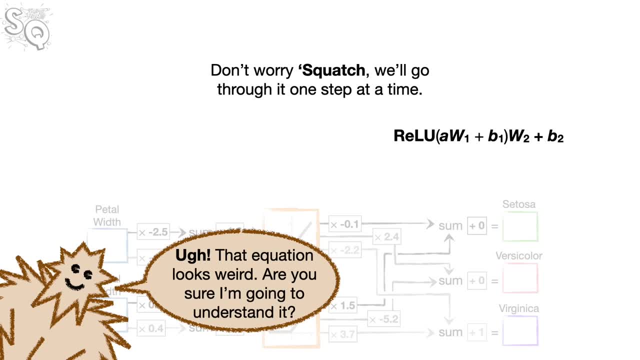 Don't worry, Squatch, We'll go through it one step at a time. Okay, However, we'll start by learning some basic terminology and build up an understanding of the matrix equation. So let's start by learning some basic terminology and. 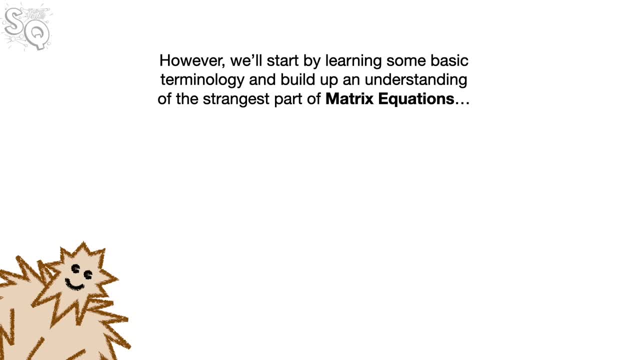 build up an understanding of the strangest part of matrix equations, Matrix multiplication. And in order to do that, imagine: StatSquatch just got a ticket to see Taylor Swift at the Friends Arena in Stockholm, Sweden. Squatch, are you ready for it? Yes, 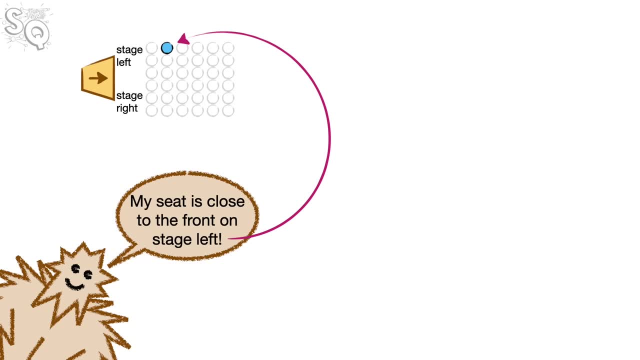 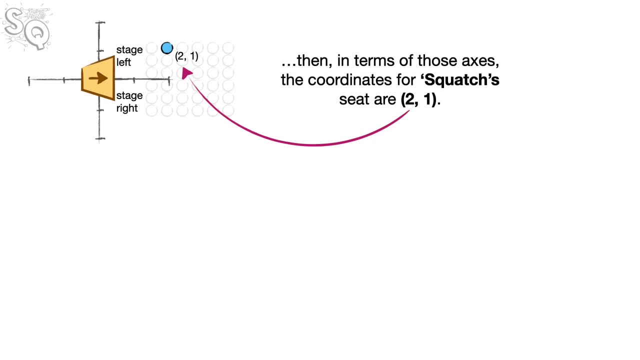 Where is your seat? My seat is close to the front on stage left. Now, if we put an x and y axis centered on the stage, Then in terms of those axes, the coordinates for Squatch's seat are 2 comma 1.. 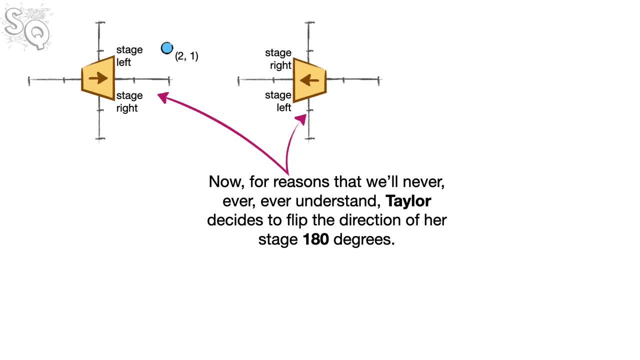 Now, for reasons that we'll never, ever, ever understand, Taylor decides to flip the direction of her stage 180 degrees. I knew she was trouble. Anyway, rotating the stage means Squatch's seat and everyone else's needs to rotate as well To determine the new x and y coordinates of Squatch's. 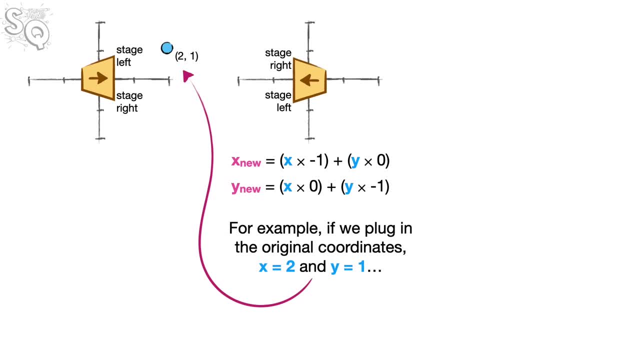 seat. we can use these equations. So let's start with the x and y coordinates of Squatch's seat. For example, if we plug in the original coordinates x equals 2 and y equals 1, then the new x and y coordinates are negative 2 comma, negative 1.. In other words, these two. 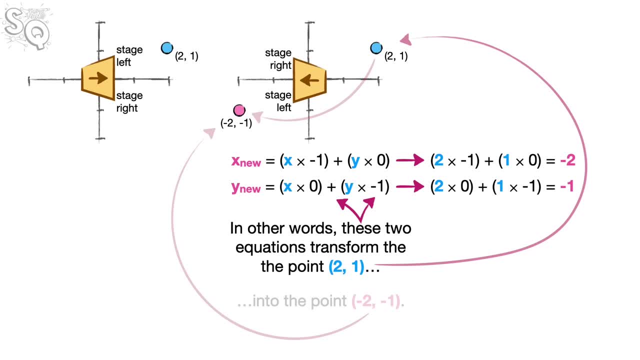 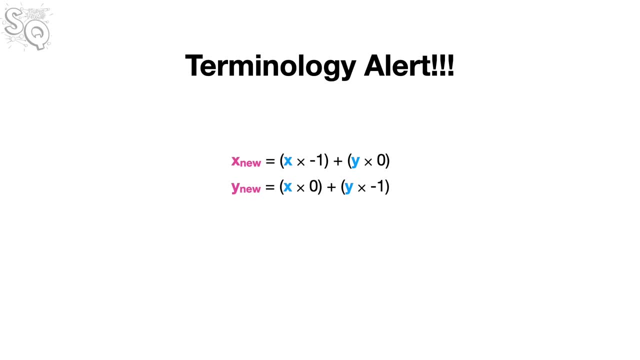 equations transform the point 2 comma 1 into the point negative 2 comma negative 1.. Oh no, it's the dreaded terminology alert, Because these equations which transform the original x and y coordinates into new x and y coordinates only multiply and add stuff to the original. 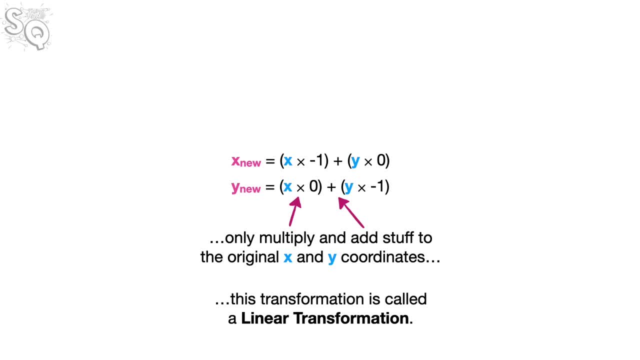 x and y coordinates. this transformation is called a linear transformation. For example, if we focus on the first equation and plug in x equals 2 and y equals 1, then we get negative 2.. If we then increase x to 3, then we get negative 3.. 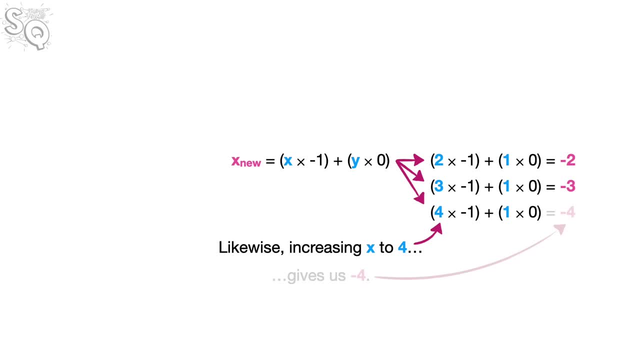 Likewise, increasing x to 4 gives us negative 4.. Thus, each time we increase the value for x by 1, we decrease the output by negative 1.. In other words, a constant change in the value for x results in a constant change in the. 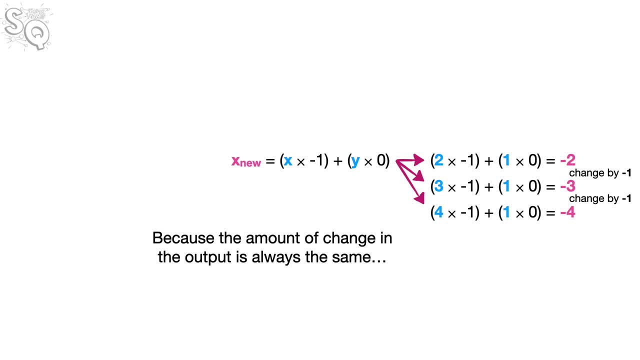 output, Because the amount of change in the output is always the same, just like the slope or the amount of change in the y-axis of a straight line is always the same. this transformation is called a linear transformation. In contrast, if the transformation was 2 to the x, then plugging in x equals 2 would give us 4,. 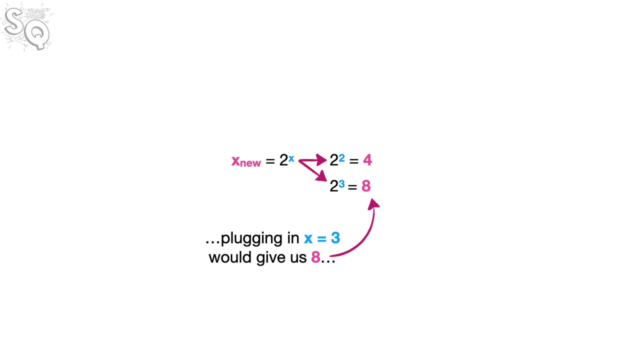 plugging in x equals 3 would give us 8, and plugging in x equals 4 would give us 16.. And we see that each time we increase the value for x by 1, the output increases by a different amount, Because 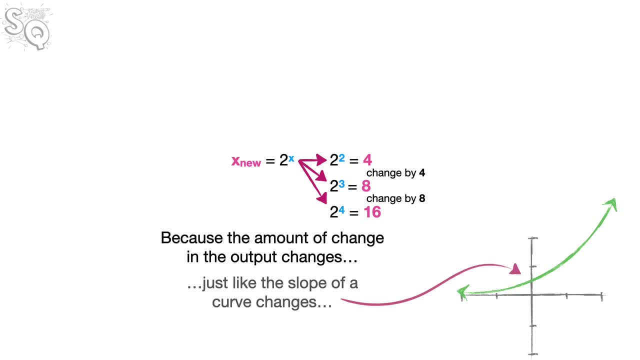 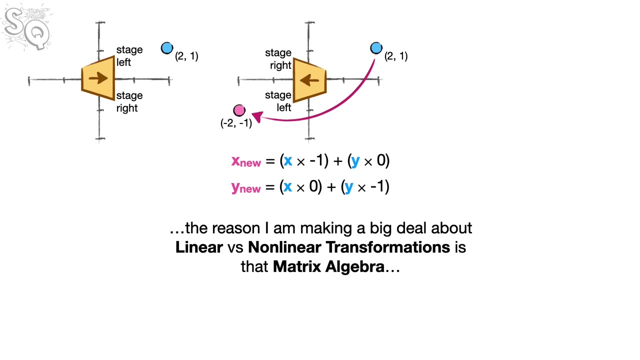 the amount of change in the output changes, just like the slope of a curve changes. this transformation is called a nonlinear transformation. Anyway, going back to our original linear transformations, the reason I'm making a big deal about linear versus nonlinear transformations is that matrix algebra 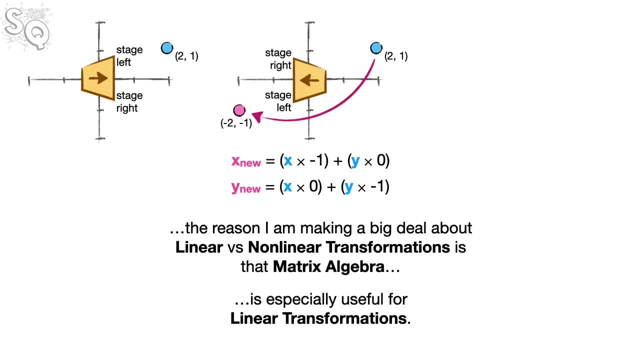 is a special function of linear transformation. It's a function of linear contributions and especially useful for linear transformations. Thus, usingping 0x, we can write out our linear transformation like this: In this example, we've put the old x and y co் into something called a row matrix or row vector. We 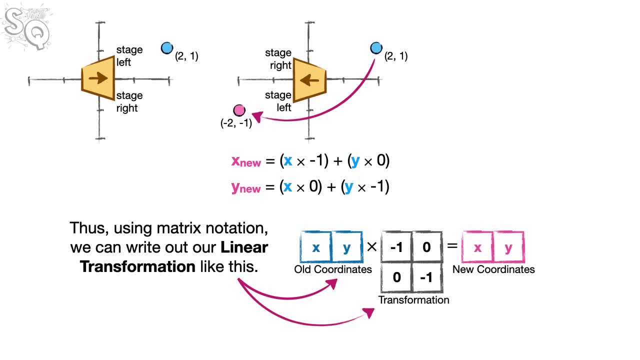 can also call this row matrix a 1 x 2 matrix, because it has 1 row and 2 numbers. 1 x 2 matrix because it has 1 row and 2 numbers. lorsque vamosStick 0x onto the matrix, so we say it has 2 columns, We can also call the matrix a row. 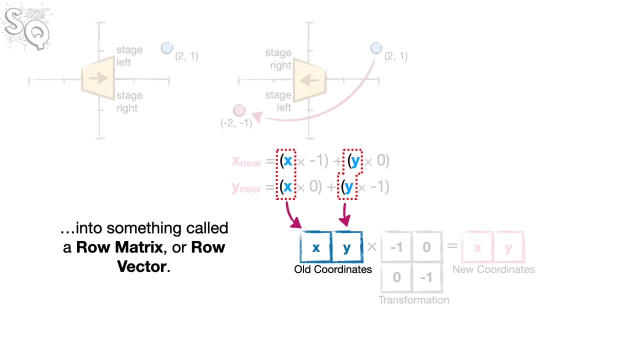 so we can say it has 1 bar. what would be the matrix of the row with larger Bet Δ? and let's say it's清 keeps 10 Zurich, so we can use that polys to remove the gap~. Amριğo bu, Another simple way to define the matrix X9!. 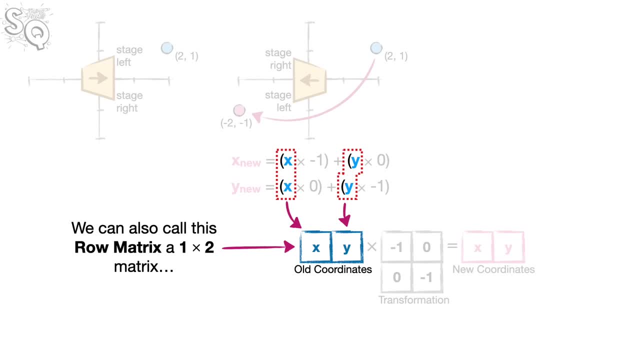 It's called a short matrix. matrix because it's long, but no long can describe the matrix as a row. The vector a helps you to make by two matrix because it has one row and two numbers in that row. so we say it has two columns. 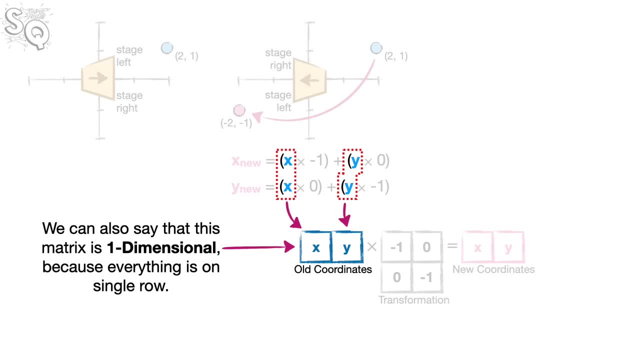 We can also say that this matrix is one-dimensional because everything is on a single row. The coefficients, the numbers we multiply x and y by and define the transformation, go into a matrix And we can call this a two by two matrix because it has two rows and two columns. 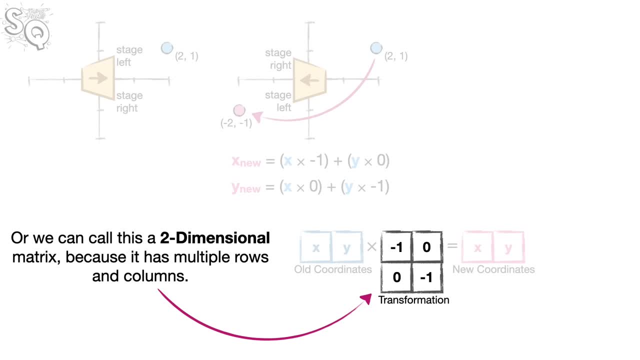 Or we can call this a two-dimensional matrix, because it has multiple rows and columns. The coefficients in the first equation go into the first column in the matrix and the coefficients in the second equation go into the second column in the matrix. Josh, this seems really weird and I have no idea how I'll remember this. 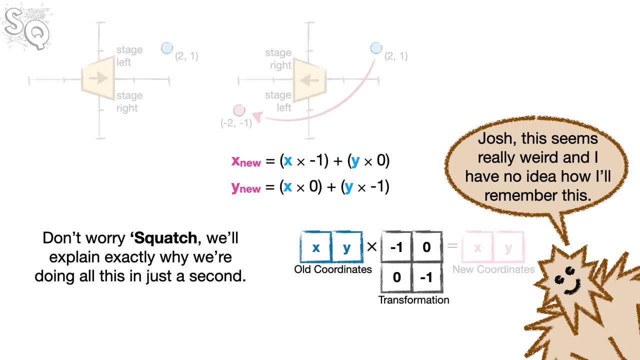 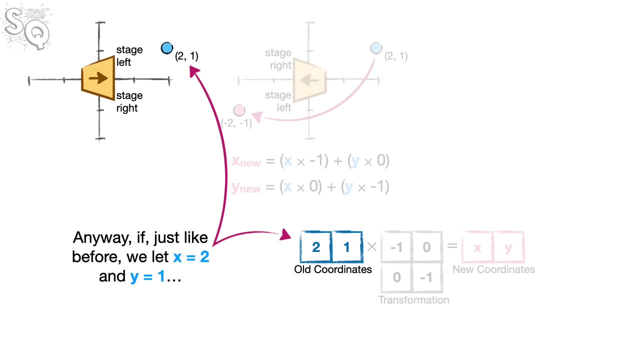 Don't worry, Squatch, We'll explain exactly why we're doing all this in just a second, And knowing why we do this will help you derive it on your own BAM. Anyway, if, just like before, we let x equal 2 and y equal 1,, 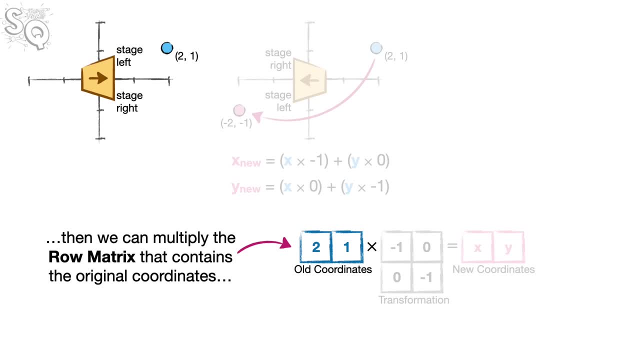 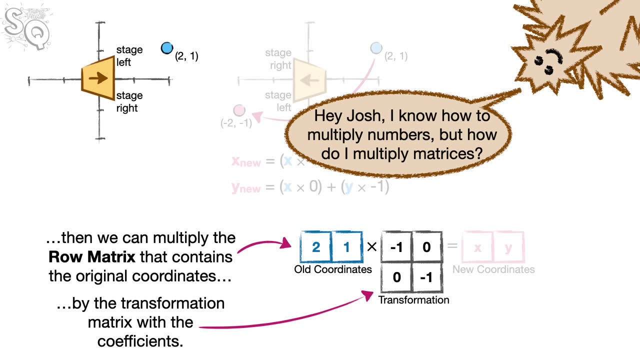 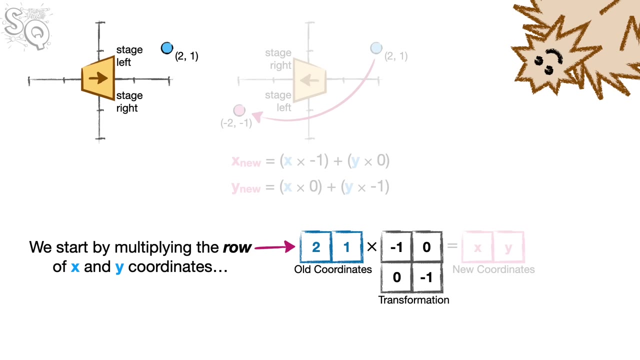 then we can multiply the row matrix that contains the original coordinates by the transformation matrix with the coefficients. Hey, Josh, I know how to multiply numbers, but how do I multiply matrices? We start by multiplying the row of x and y And by multiplying the row of x and y coordinates. 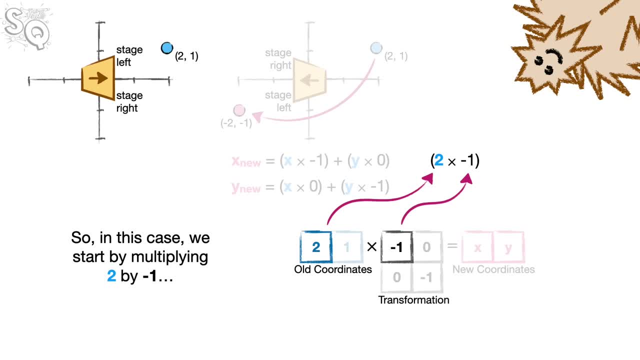 by the numbers in the first column in the transformation matrix. So in this case we start by multiplying two by negative one, Then we multiply one by zero And lastly we add the terms together And this gives us the original transformation for the new x coordinate that we started with. 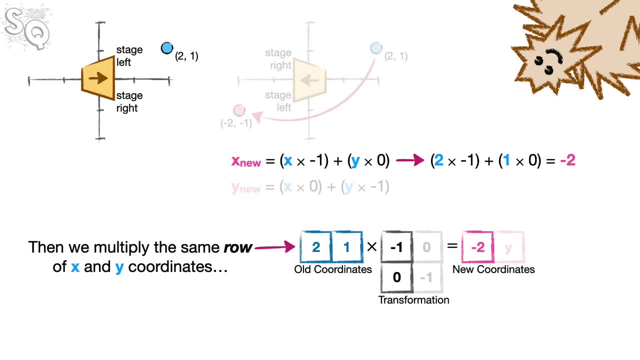 which tells us that the new x coordinate is negative 2. the same row of x and y coordinates by the numbers in the second column in the transformation matrix. So that means we multiply 2 by 0 and 1 by negative 1.. And 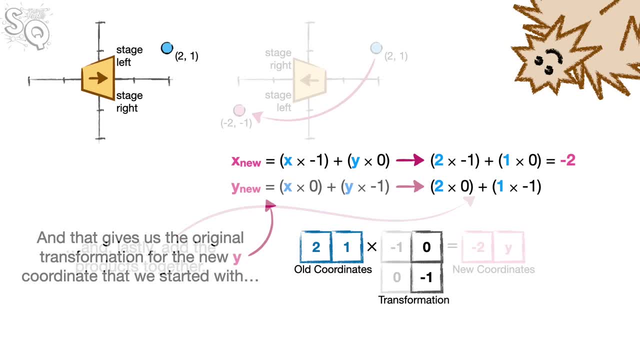 lastly, add the products together And that gives us the original transformation for the new x coordinate that we started with, which tells us that the new y coordinate is negative. 1. Combined, the matrix multiplication transforms the old x and y coordinates to the new x and y coordinates. 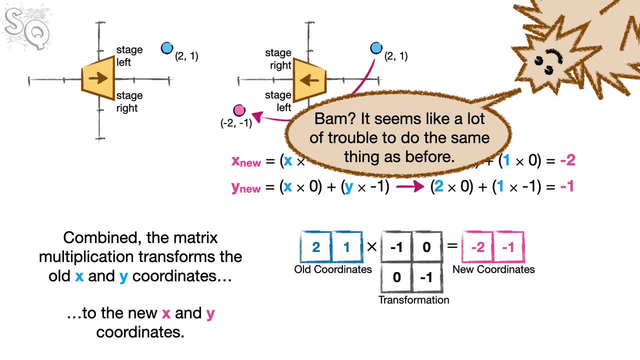 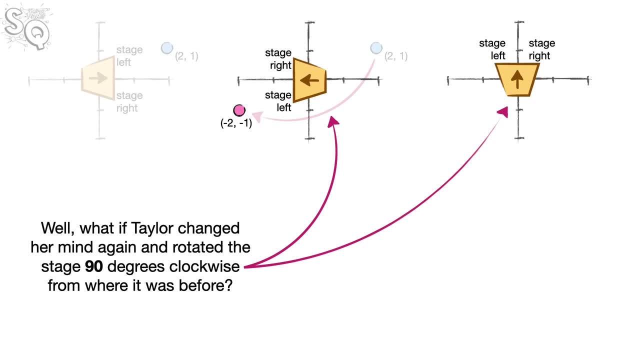 Bam. It seems like a lot of trouble to do the same thing as before. Well, what if Taylor changed her mind again and rotated the stage 90 degrees clockwise from where it was before? Oops, she did it again. No Squatch. 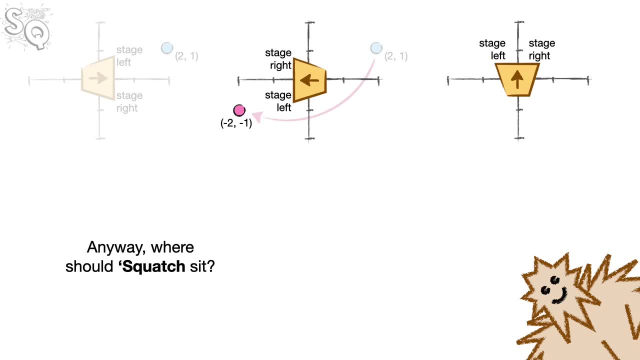 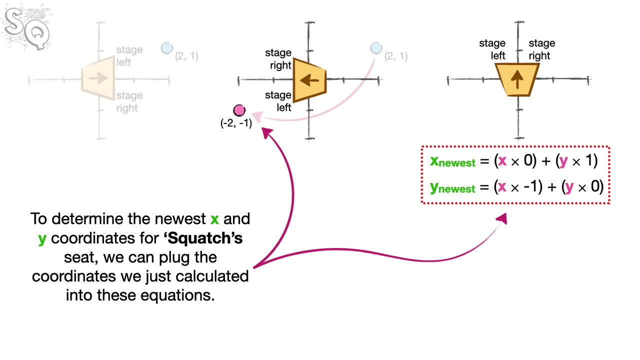 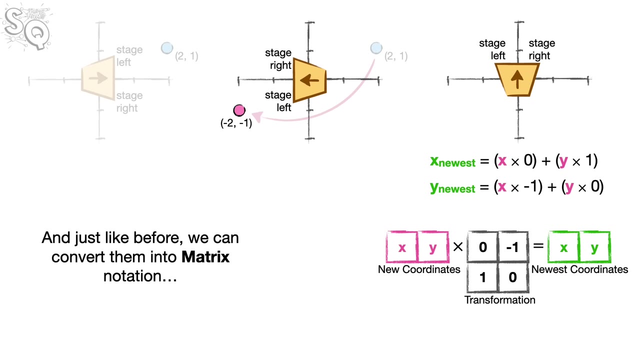 That's not what I meant. That's Britney Spears. Anyway, where should Squatch sit? To determine the newest x and y coordinates for Squatch's seat, we can plug the coordinates we just calculated into these equations And, just like before, we can convert them into matrix notation by putting the x and 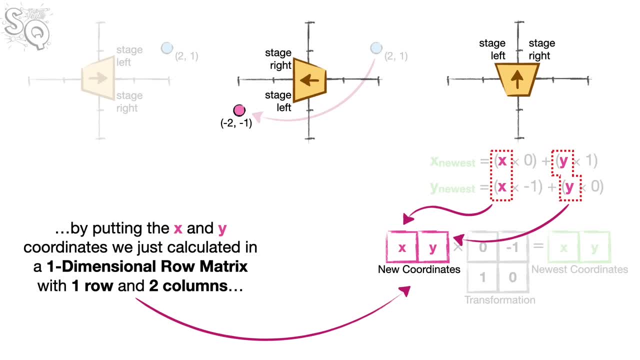 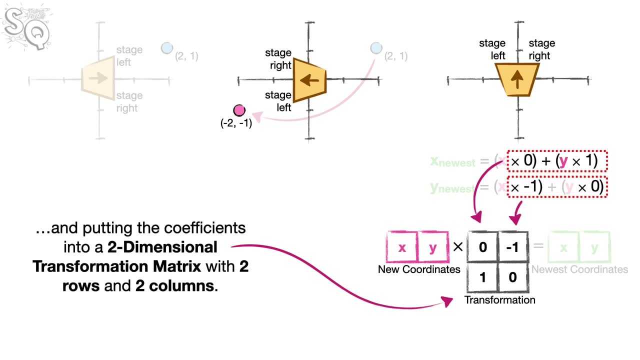 y coordinates. we just calculated in a one-dimensional row matrix with one row and two columns and putting the coefficients into a two-dimensional transformation matrix with two rows and two columns, The coefficients in the first equation go into the first column in the transformation matrix And the coefficients in the second equation go into the second. 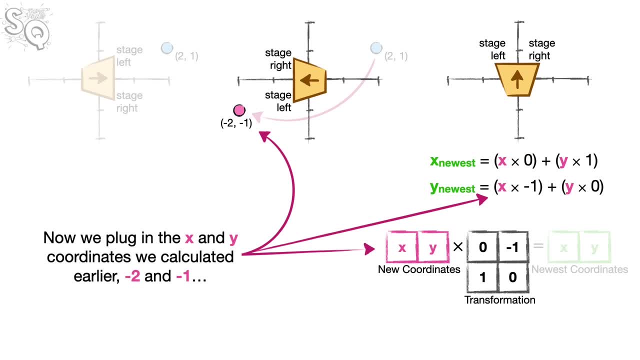 column in the transformation matrix. Now we plug in the x and y coordinates we calculated earlier – negative 2 and negative 1.. And do the matrix multiplication just like before – row by column. We start by multiplying the row of x and y coordinates with the first. 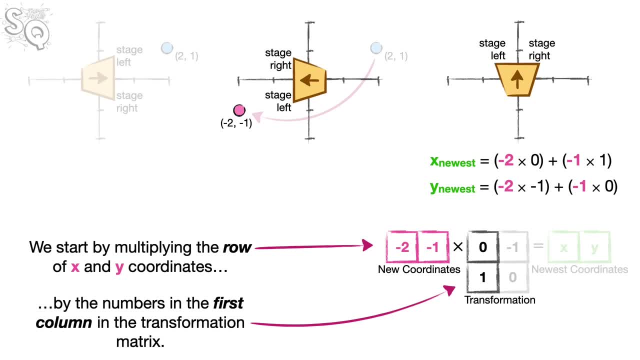 coordinates by the numbers in the first column in the transformation matrix. So we multiply negative 2 by 0 and we multiply negative 1 by 1, and then we add the terms together and that gives us the newest x coordinate, negative 1.. Then we 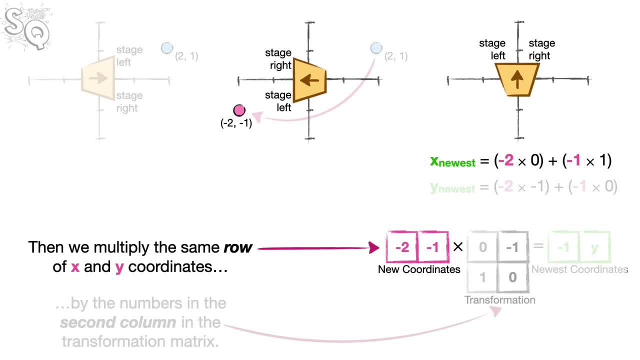 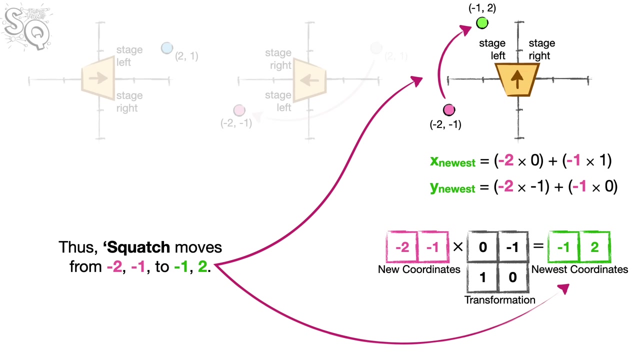 multiply the same row of x and y coordinates by the numbers in the second column in the transformation matrix. So we multiply negative 2 by negative 1 and multiply negative 1 by 0, and then add the terms together. That gives us the newest y coordinate 2.. Thus Squatch moves from negative 2 comma negative 1 to 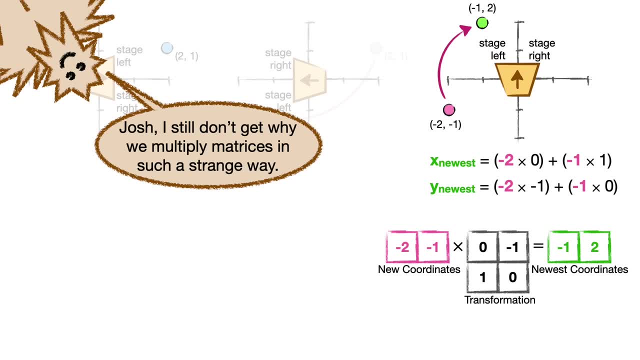 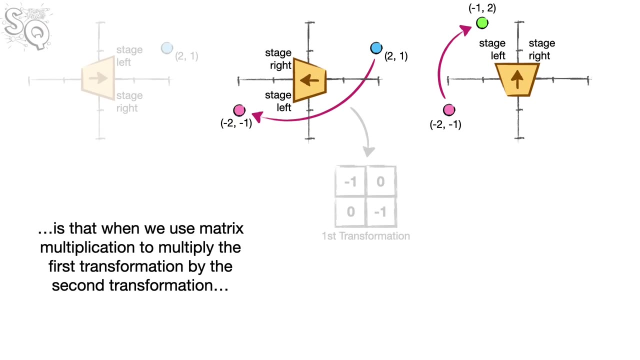 negative 1 comma 2.. Josh, I still don't get why we multiply matrices in such a strange way. Well, the reason is that we multiply the numbers in a row by the numbers in a column and then add the products together. is that when we use matrix multiplication to multiply the first? 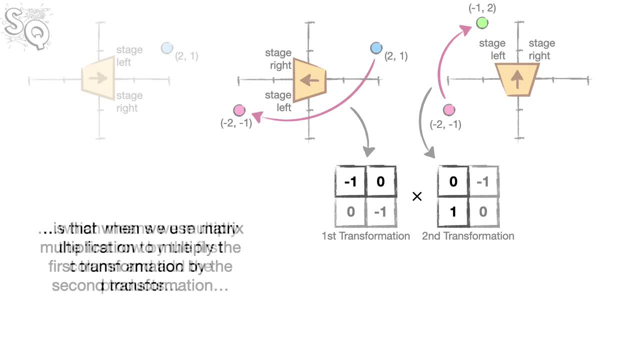 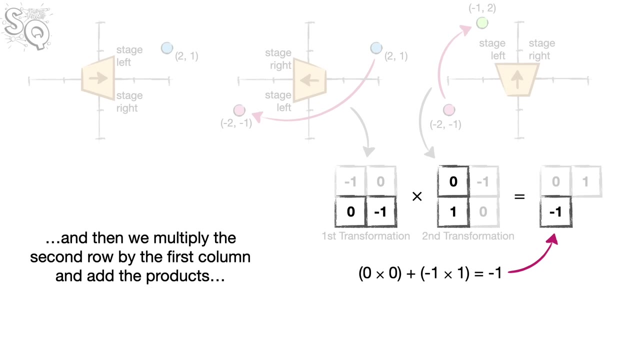 transformation by the second transformation, which means we multiply the first row by the first column and add the products, and we multiply the first row by the second column and add the products, and then we multiply the second row by the first column and add the products. 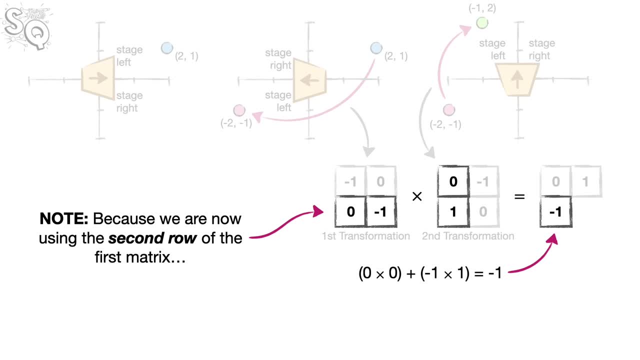 note, because we are now using the second row of the first matrix, we put the result in the second row in the output. In other words, when we use a new row to do multiplication, we start a new row in the output matrix. Anyway, then we 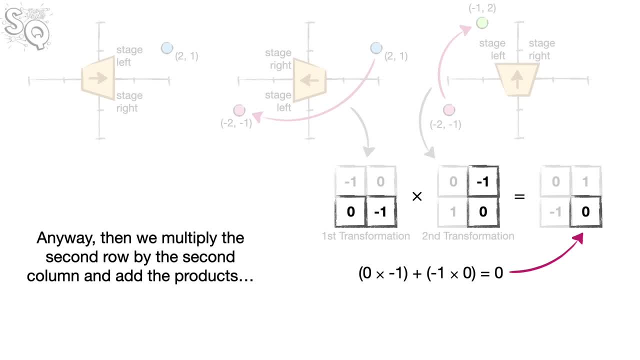 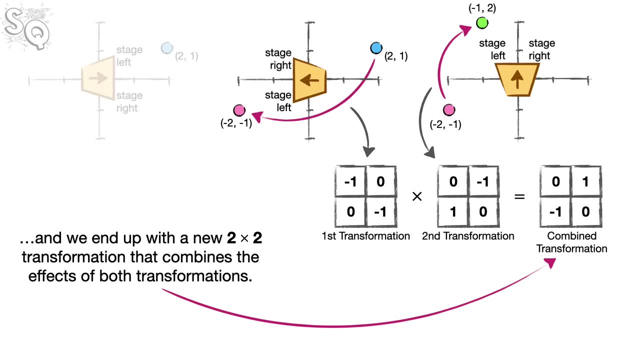 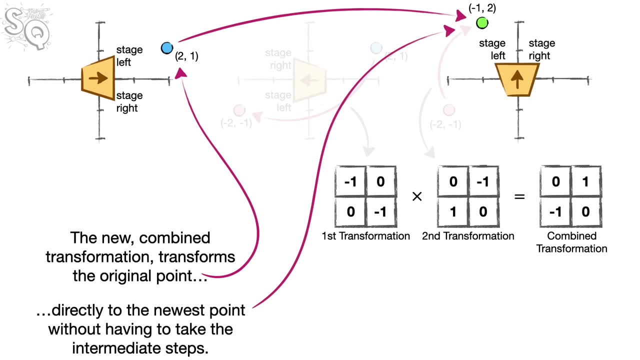 multiply the second row by the second column and add the products and we end up with a new 2 by 2 transformation that combines the effects of both transformations. The new combined transformation transforms the original point directly to the newest point without having to take the intermediate steps, In other words matrix. 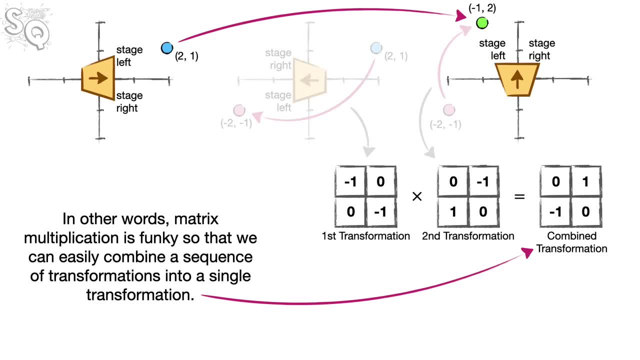 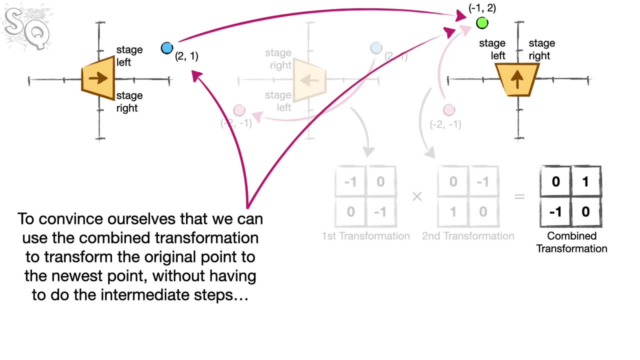 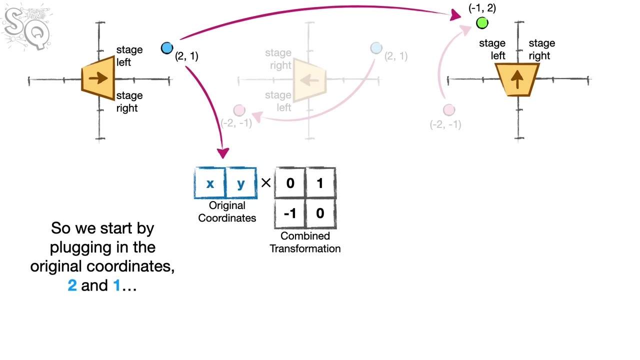 multiplication is funky, so that we can easily combine a sequence of transformations into a single transformation. To convince ourselves that we can use the combined transformation to transform the original point to the newest point without having to do the intermediate steps, let's multiply the original coordinates by the combined transformation. So we start. 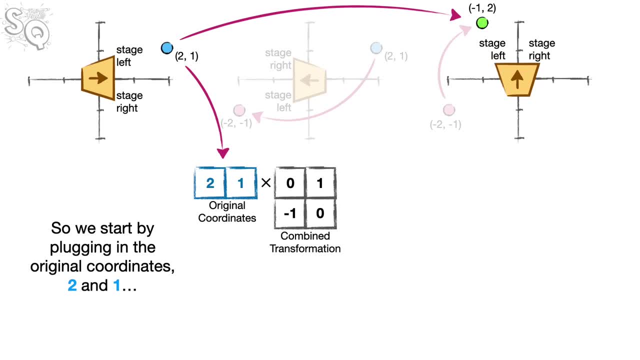 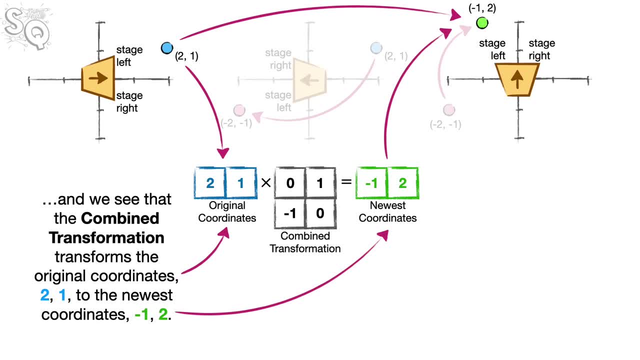 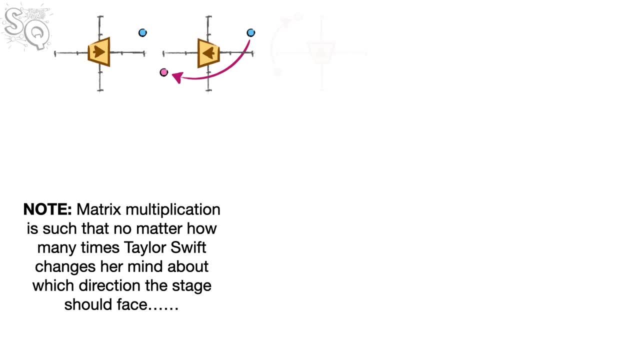 coordinates 2,1 to the newest coordinates negative, 1,1.. 2. BAM Matrix multiplication is such that, no matter how many times Taylor Swift changes her mind about which direction the stage should face, we can just multiply the individual transformations together to get a. 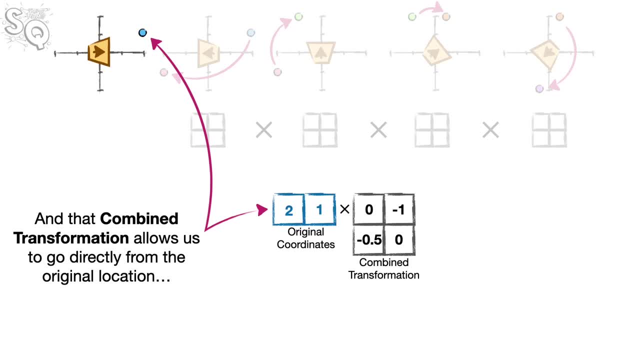 combined transformation. And that combined transformation allows us to go directly from the original location to the final location without having to do the intermediate steps, BAM. Okay, now that we understand why matrix multiplication is so funky, let's talk about another confusing thing, about. 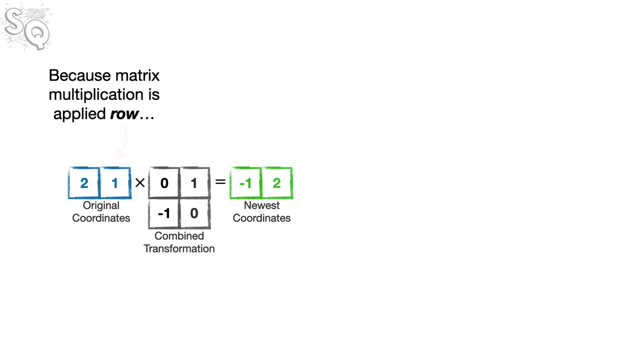 matrix multiplication. Because matrix multiplication is applied row by column, we can't just reverse the order of the matrices and expect things to work out the same. In fact, we can't even multiply these two matrices together, because each row in the first matrix has two numbers and each column in the second. 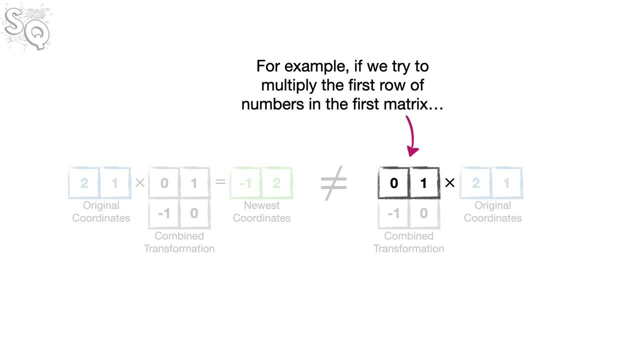 matrix only has one number. For example, if we try to multiply the first row of numbers in the first matrix by the first column of numbers in the second matrix, then we can multiply 0 by 2, but there is nothing to multiply this 1 by In. 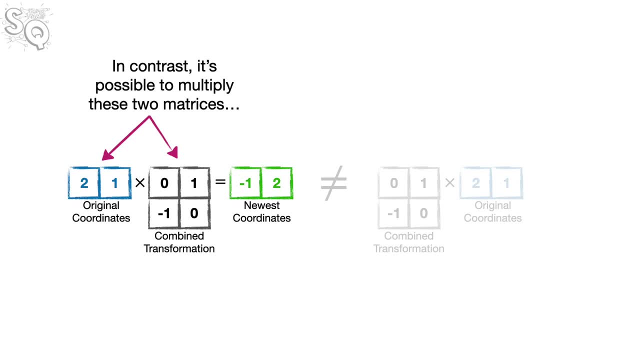 contrast, it's possible to multiply these two matrices because we have the same number of values in this row that we have in these columns. In general, the number of columns in the first matrix has to match the number of rows in the second matrix. If, for some reason, we want to switch the order of these matrices, then 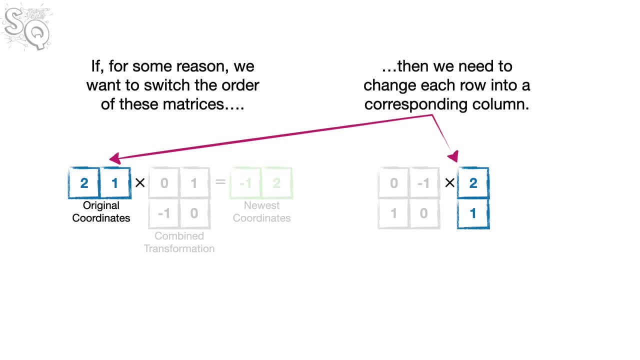 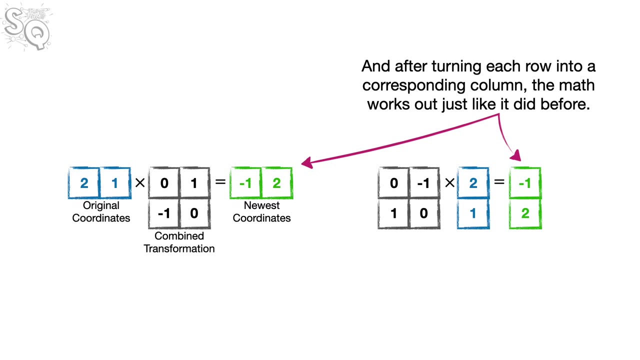 we need to change each row into a corresponding column. Now we can do the multiplication correctly, row by column, And after turning each row into a corresponding column, the math works out just like it did before- Note, because we turned the rows in the original matrices. 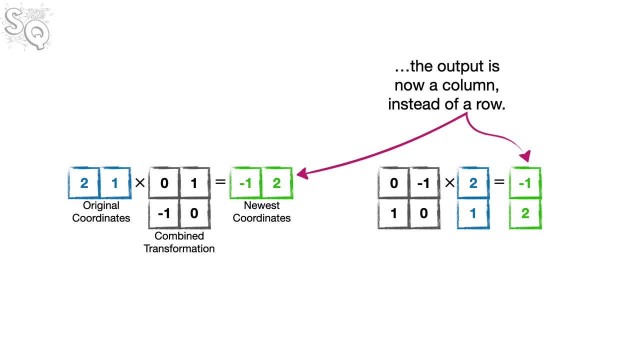 into columns. the output is now a column instead of a row. Oh no, it's the dreaded terminology alert. Changing the rows in a matrix into corresponding columns is called transposing a matrix, and we notate the transpose function with a superscript function. 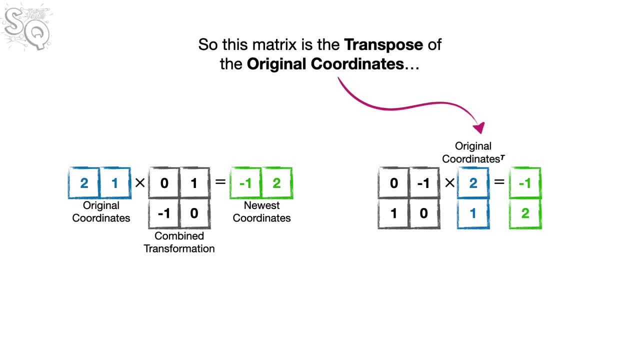 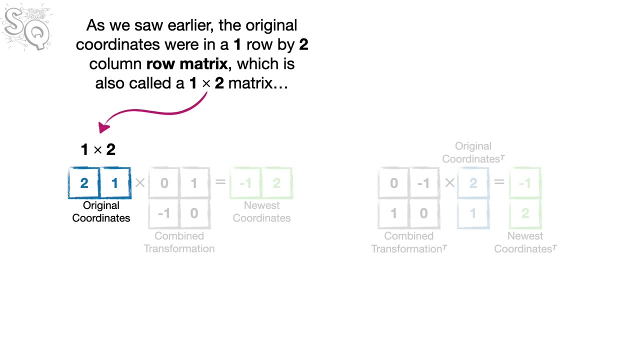 So this matrix is the transpose of the original coordinates, This is the transpose of the combined transformation matrix And this is the transpose of the newest coordinates. As we saw earlier, the original coordinates were in a one row by two column row matrix, which is also called a 1 by 2 matrix. But after we 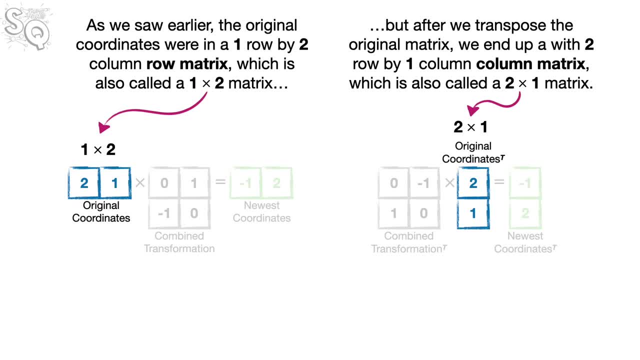 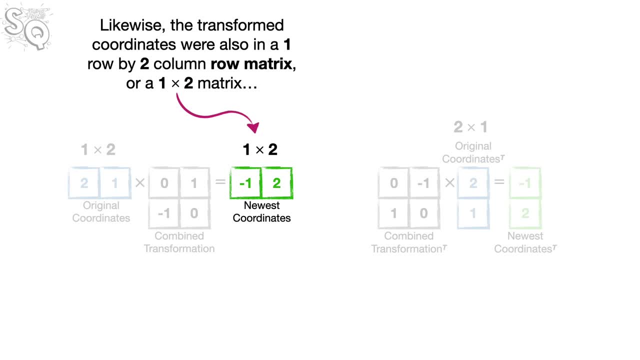 transpose the original matrix, we end up with a two row by one column column matrix, which is also called a 2 by 1 matrix. Likewise, the transformed coordinates were also in a one row by two column row matrix or a one by two. 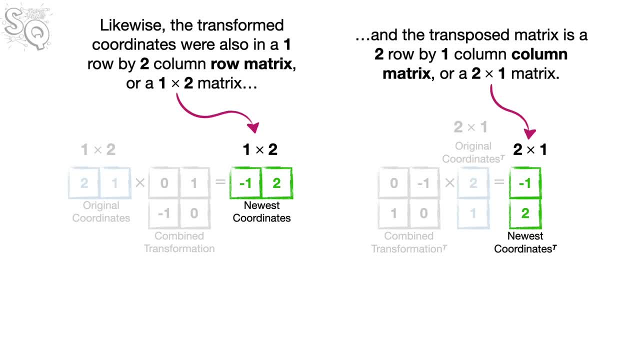 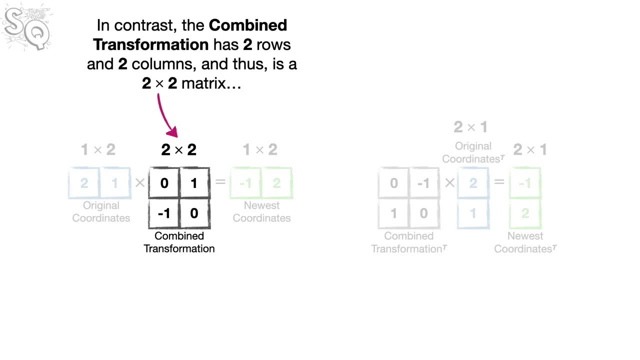 matrix And the transposed matrix is a two row by one column column matrix or a two by one matrix. In contrast, the combined transformation has two rows and two columns and thus is a two by two matrix And the transposed matrix also. 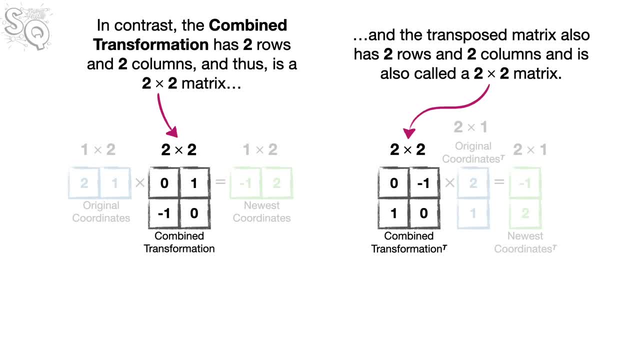 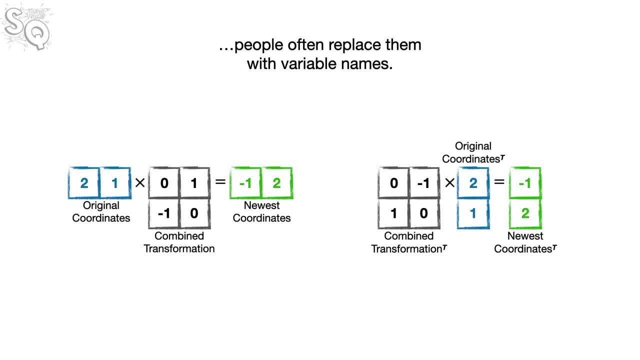 has two rows and two columns and is also called a 2x2 matrix. Now, because writing out matrices can be cumbersome, people often replace them with variable names. Matrices with only one row or column are usually referred to with lowercase letters, that are sometimes italicized and sometimes not, and 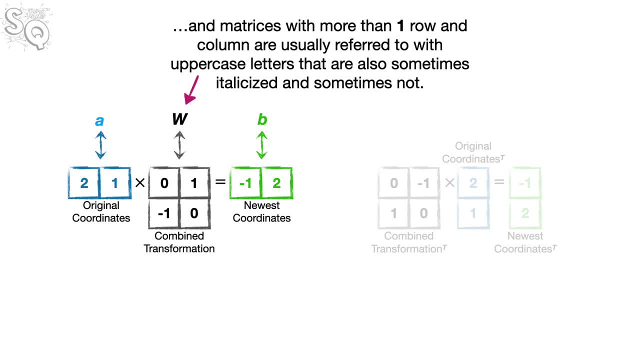 matrices with more than one row and column are usually referred to with uppercase letters. that are also sometimes italicized and sometimes not. Out in the wild you'll find additional notation styles, so just be prepared to be flexible. Anyway, given these variable names, we can rewrite the matrix equation. 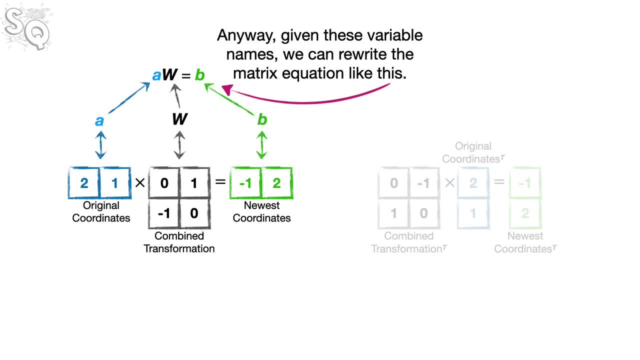 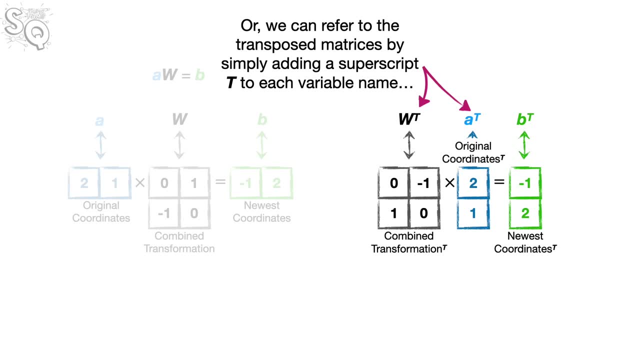 like this: A times W equals B. Or we can refer to the transposed matrices by simply adding a superscript T to each variable name and rewrite the matrix equation as follows. Like this: The transpose of W times the transpose of A equals the transpose of B. 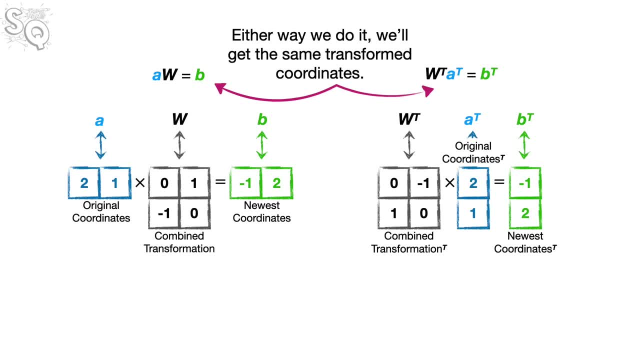 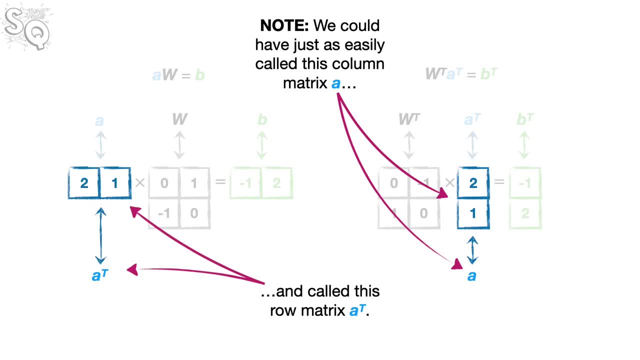 Either way we do it, we'll get the same transformed coordinates. Note: we could have just as easily called this column matrix A and called this row matrix the transpose of A. Likewise, we could call this matrix W and this matrix the transpose of W. Lastly, this column matrix is called the transpose of A. 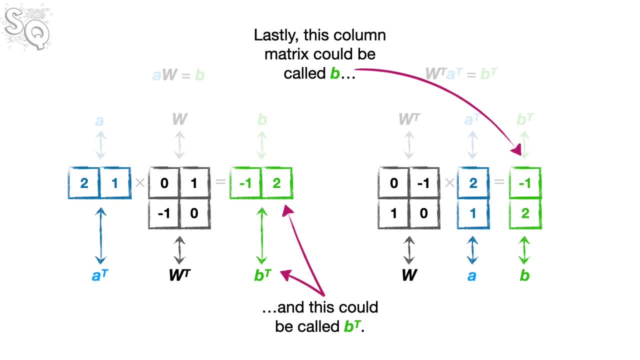 This column matrix could be called B and this could be called the transpose of B. Thus we could also write the matrix equations like these: The transpose of A times the transpose of W equals the transpose of B, or W times A equals B. I mentioned these alternative ways to write the equations because out 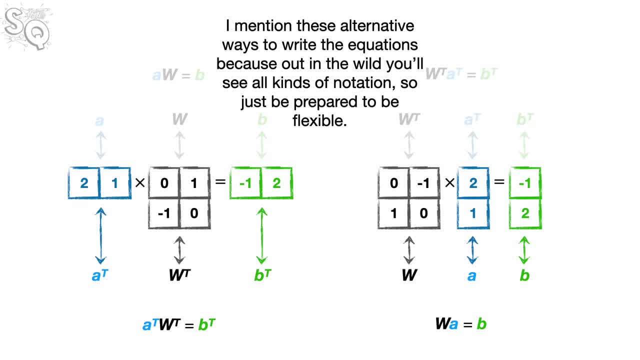 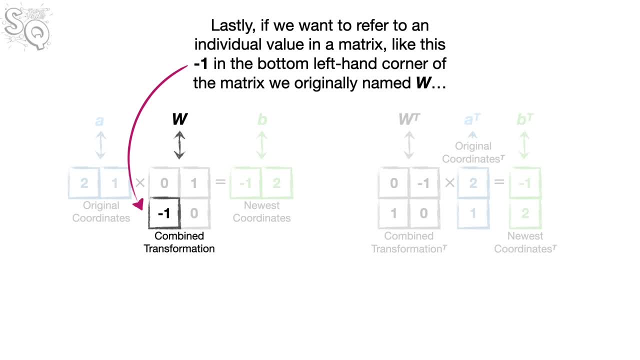 to refer to an individual value in a matrix like this: negative 1 in the bottom left-hand corner of the matrix we originally named W. Then if the variable is uppercase, we convert it to lowercase and add subscript, row and column indices like this: 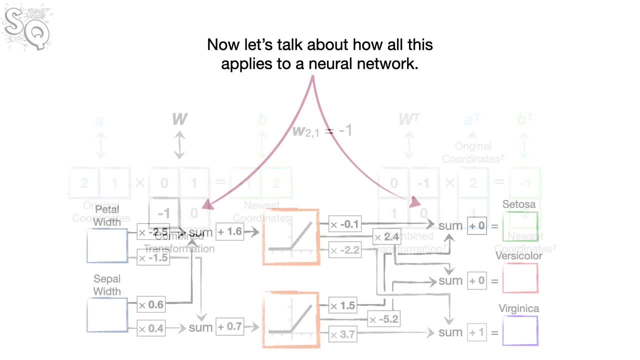 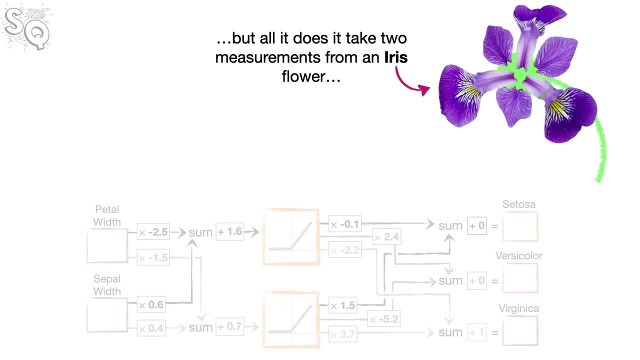 Bam. Now let's talk about how all this applies to a neural network. This neural network may look really fancy, but all it does is take two measurements from an iris flower: the width of a petal, which is this part of the flower, and the width of a sepal, which is this. 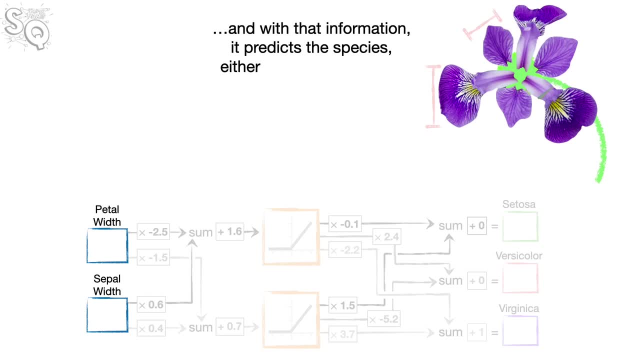 part of the flower And with that information it predicts the species: either setosa versicolor or virginica. Anyway, let's start with a petal that is 0.5 units wide and a sepal that is 0.4. 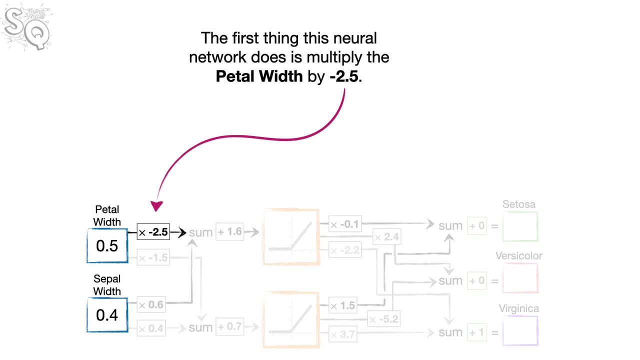 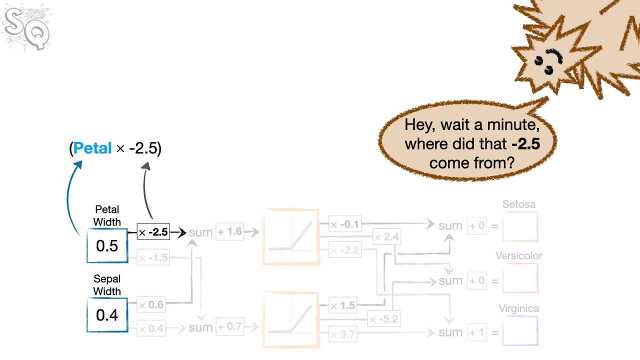 units wide. The first thing this neural network does is multiply the petal width by negative 2.5.. Hey, wait a minute. where did that negative 2.5 come from? All of the numbers in this, and pretty much every neural network, come from something called back. 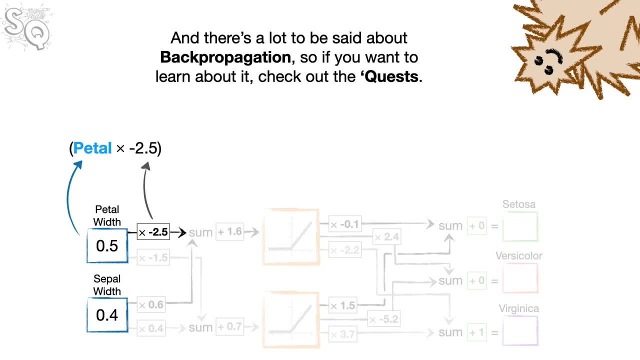 propagation, And there's a lot to be said about back propagation. so if you want to learn about it, check out the quests. Anyway, then we add that term to the sepal width multiplied by 0.5.. Then we add that term to the sepal width multiplied by 0.6.. And at the same time, 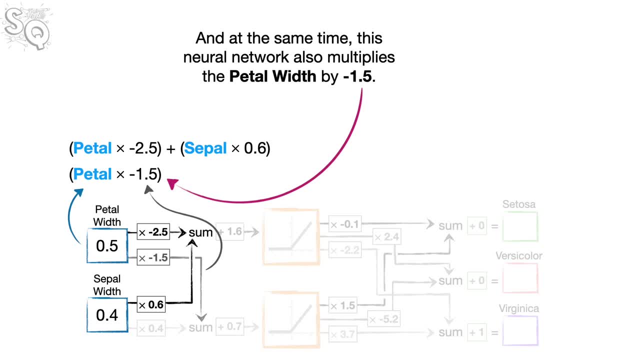 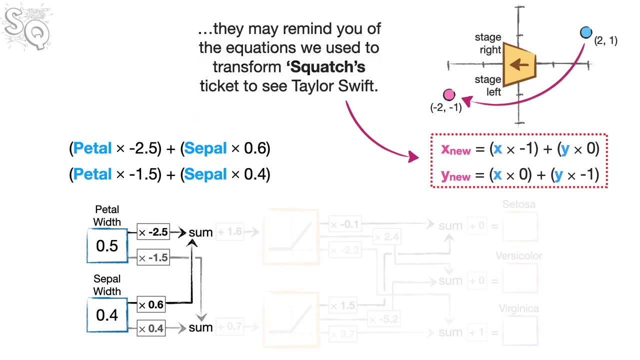 this neural network also multiplies the petal width by negative 1.5. Then we add that term to the sepal width multiplied by 0.4.. Now, even though we are looking at these equations for the first time, they may remind you of the. 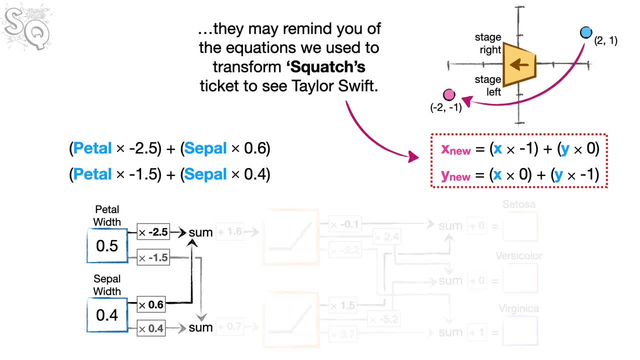 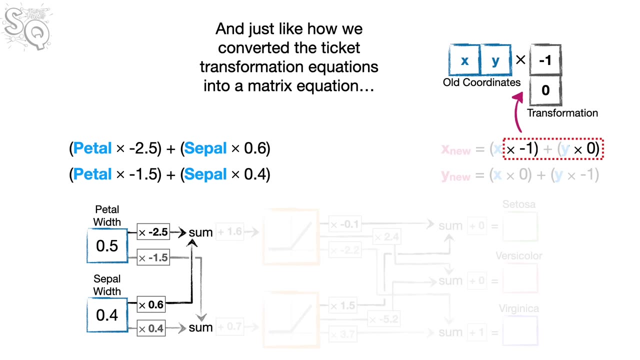 equations used to transform Squatch's ticket to see Taylor Swift. Those memories follow me around. In both cases, we have two variables multiplied by numbers and then the terms are added together, And just like how we converted the ticket transformation equations into a matrix equation. 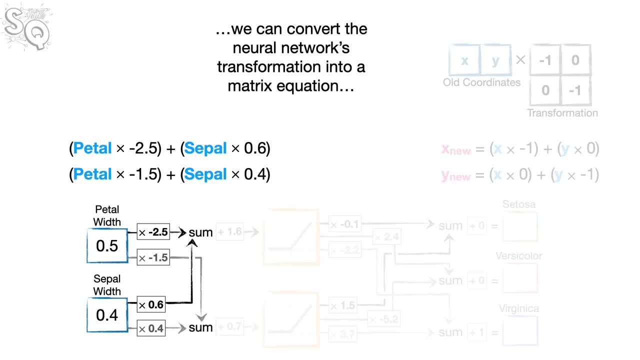 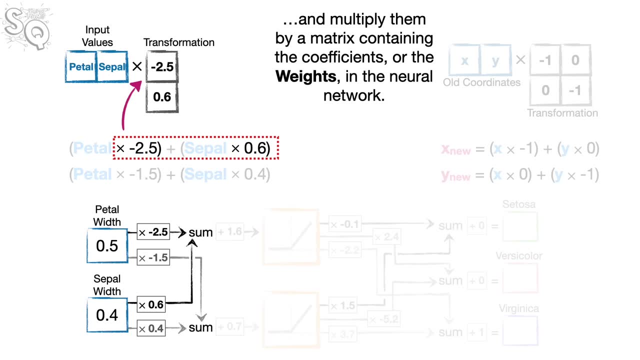 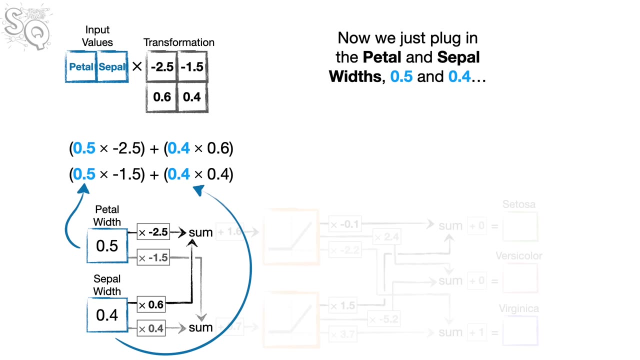 we can convert the neural network's transformation into a matrix equation where we put the petal and sepal widths into a row matrix and multiply them by a matrix containing the coefficients or the weights in a neural network. Now we just plug in the petal and 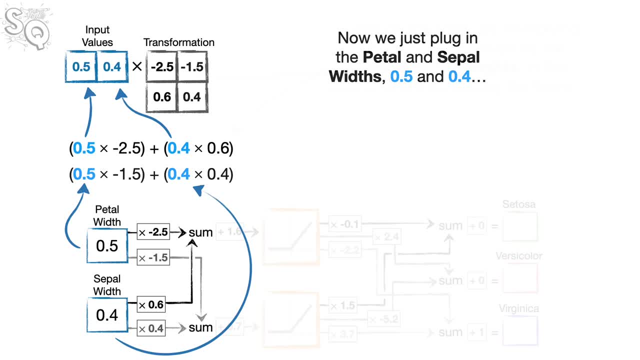 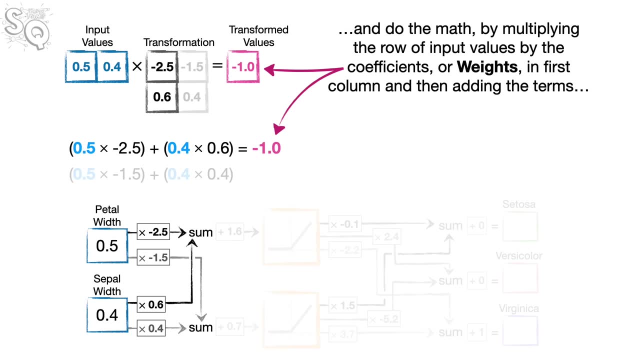 sepal widths 0.5 and 0.4, and do the math by multiplying the row of input values by the coefficients or weights in the first column and then adding the terms, And then multiplying the row of input values by the weights in the second column and then adding the terms, And that gives: 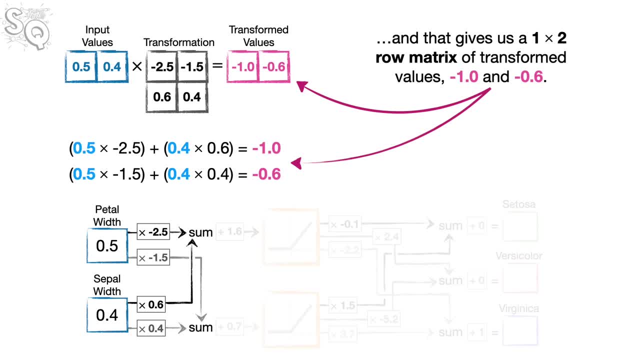 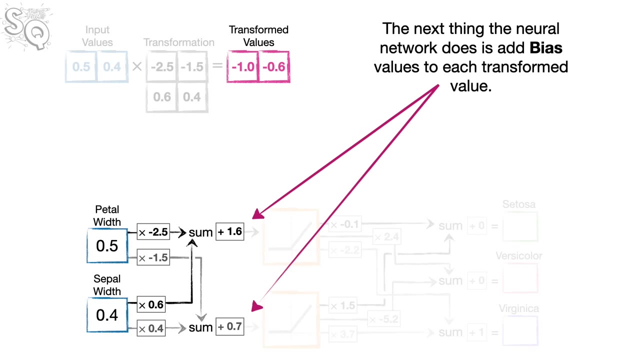 us a one by two row matrix of transformed values: negative 1.0 and negative 0.6.. So this first part of the neural network transforms the input values. The next thing the neural network does is add bias values to each transformed value. So that means we add 1.6 to the first transformed value. 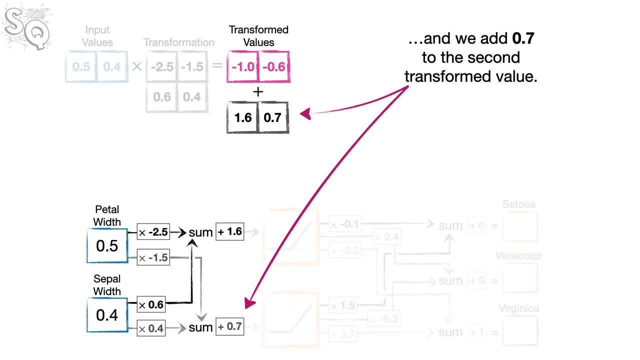 and we add 0.7 to the second transformed value And when we do the addition we end up with a row matrix with 0.6 in the first column and 0.1 in the second column. Now we are ready to use 0.6 as the x-axis coordinate for the activation function on top and 0.1 as the 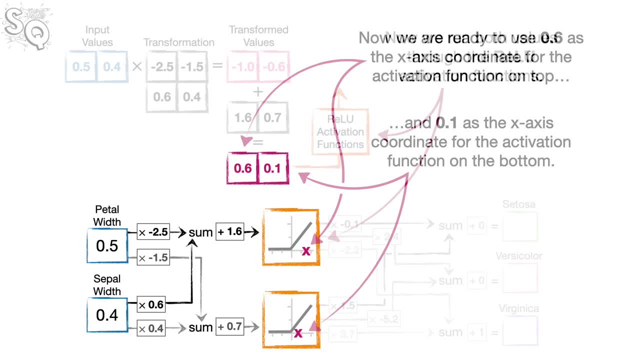 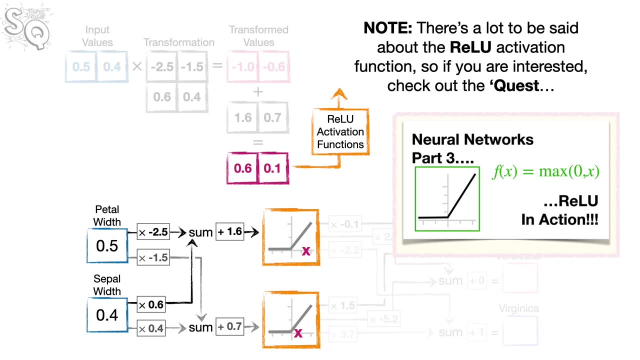 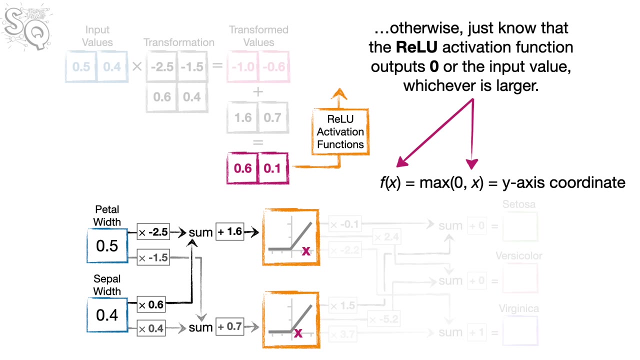 x-axis coordinate for the activation function on the bottom. Now we run both values through the rel u activation functions. Note: there's a lot to be said about the rel u activation function, so if you're interested, check out the quest. Otherwise, just know that the rel u activation 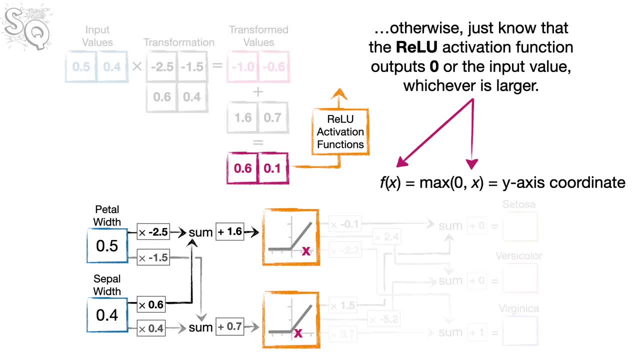 function outputs zero or the input value, whichever it is. Thus, because the input for the top rel u is 0.6,, which is greater than zero, the output is 0.6.. And because the input for the bottom rel u is 0.1,, which is also greater than zero. 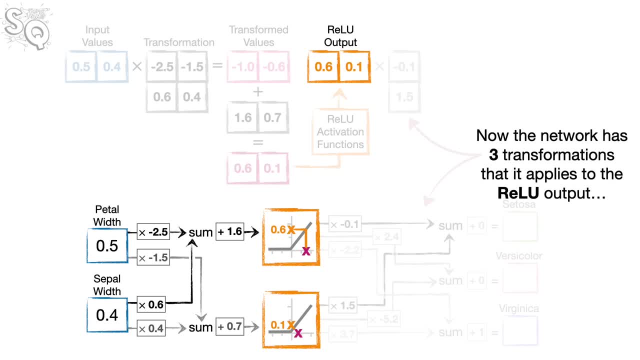 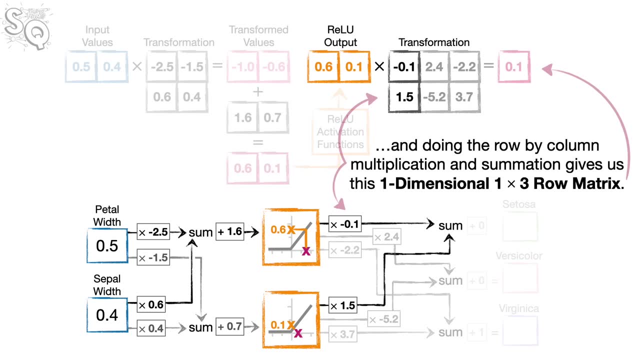 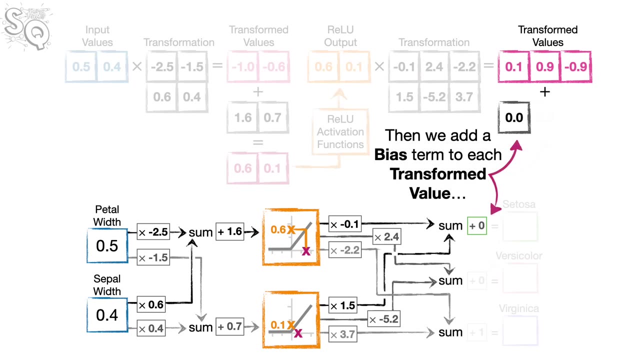 the output is 0.1.. Now the network has three transformations that it applies to the rel u output. And doing the row by column, multiplication and summation gives us this one-dimensional, one-by-three row matrix. Then we add bias terms to each transformed value. 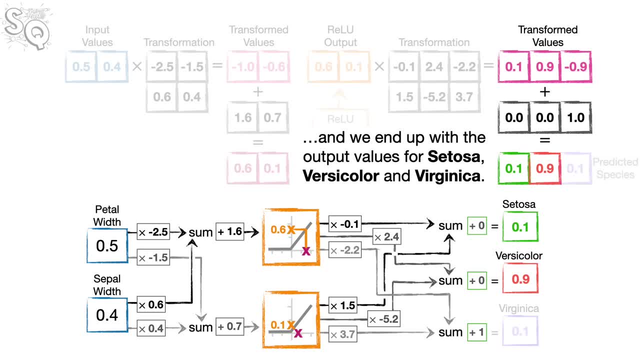 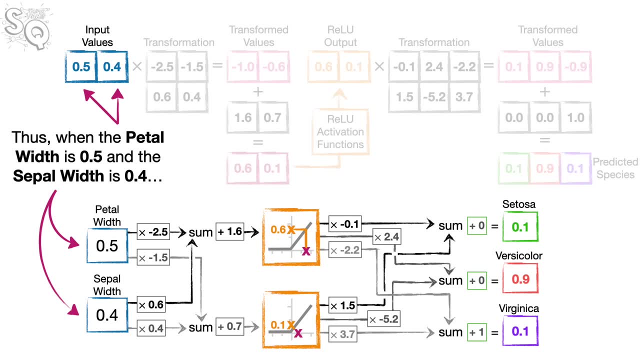 And we end up with the output values for setosa, versicolor and virginica Bam. Thus, when the petal width is 0.5 and the sepal width is 0.4,, this neural network predicts that the measurements came from versicolor, since its output value is closest to one. 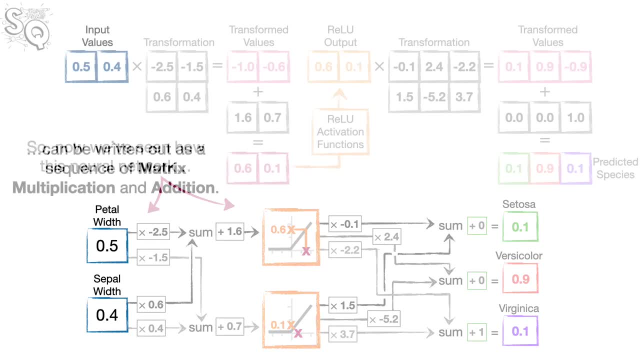 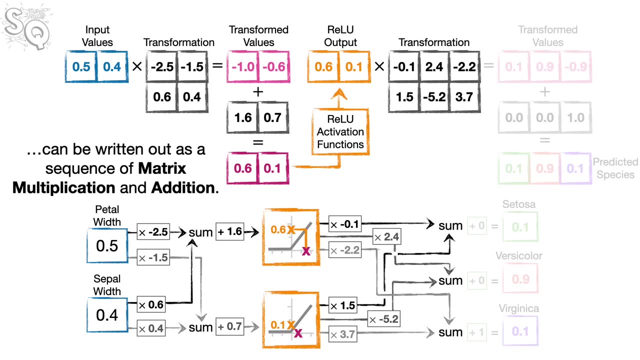 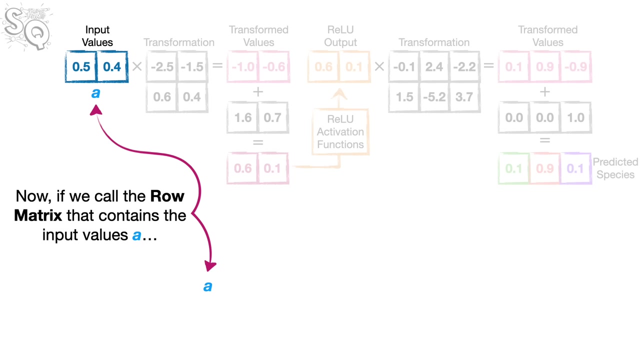 So, now that we've seen how this neural network can be written out as a sequence of matrix, multiplication and addition, Now, if we call the row matrix that contains the input values a, and we call the first transformation matrix which contains weights w sub 1.. and the first row matrix of bias terms, 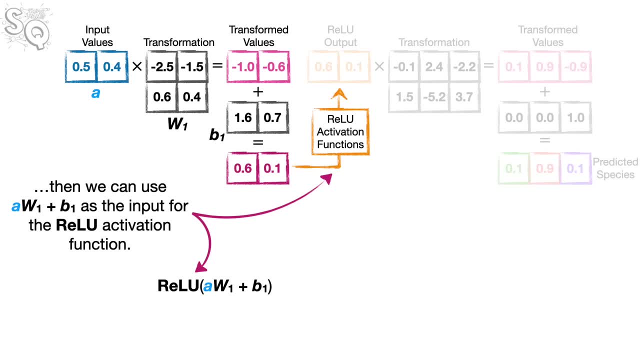 b sub 1.. then we can who Use A times W sub 1 plus B sub 1 as the input for the relu activation function. We can then multiply the output of the relu by the next transformation matrix, which we'll call W sub 2, because it also contains weights. 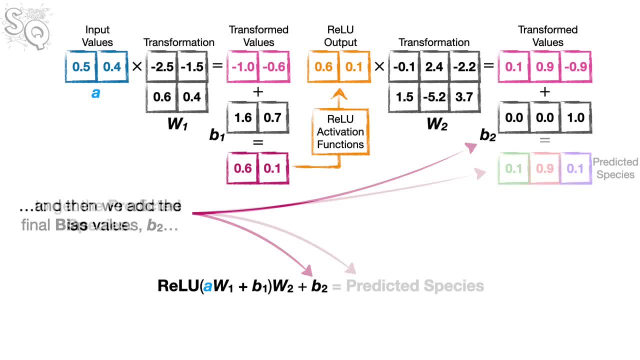 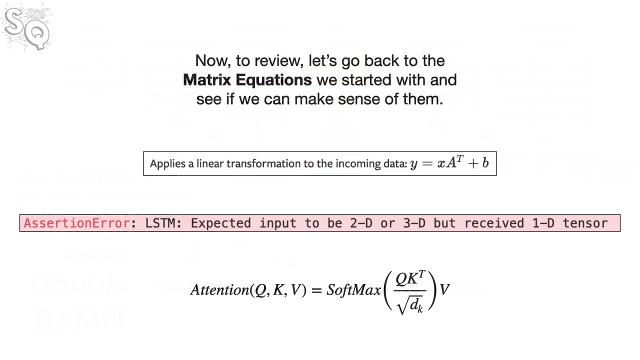 And then we add the final bias values- B, sub 2, to get the predicted species And at long last we've seen how to transform a neural network into a super compact matrix equation- Double bam. Now to review, let's go back to the matrix equations we started with and see if we can. 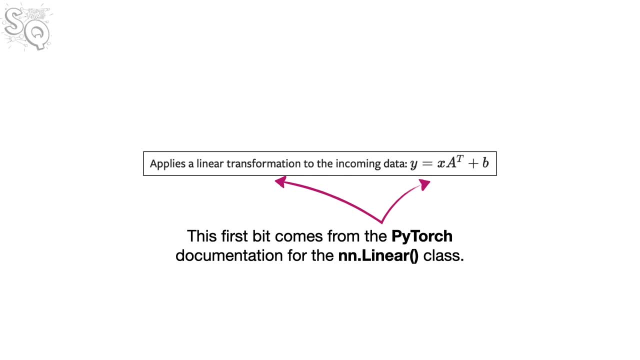 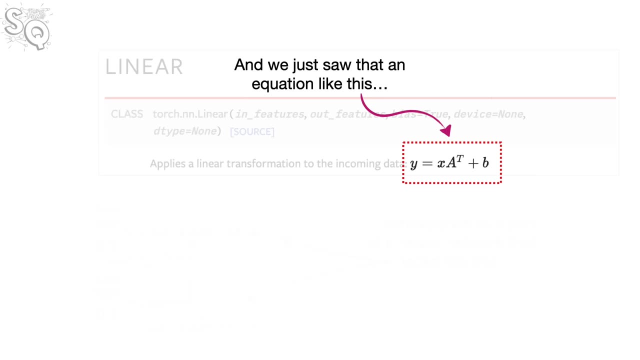 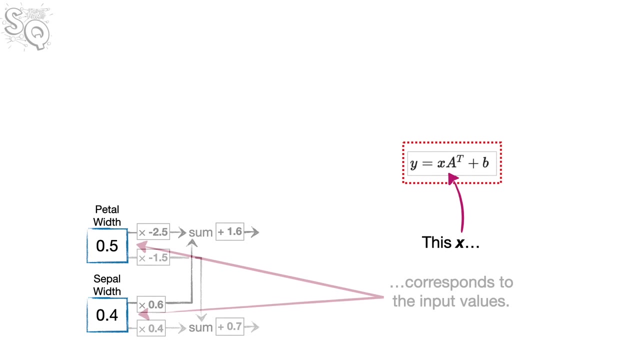 make sense of them. This first bit comes from the PyTorch documentation for the NNLinear class, And we just saw that an equation like this corresponds to a part of a neural network that looks like this: This X corresponds to the input values and, like we saw before, the input values can be. 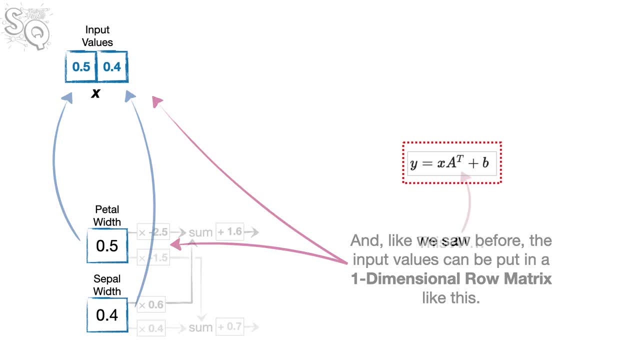 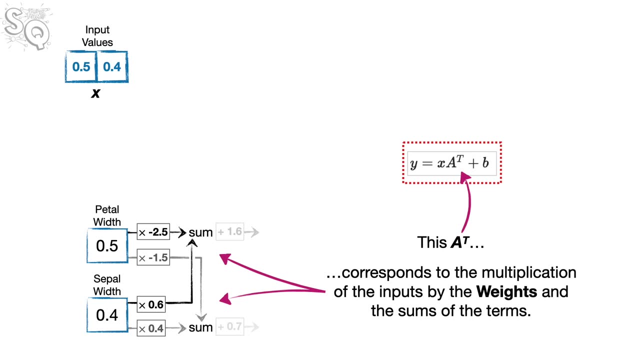 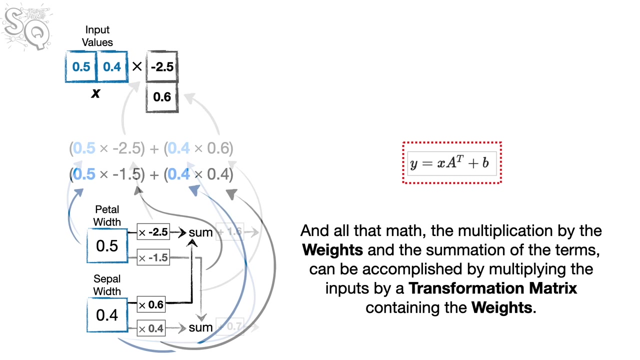 put in a one-dimensional row matrix like this. This transpose of A corresponds to the multiplication of the inputs by the weights and the sums of the terms. And all that math- the multiplication by the weights and the summation of the terms- can be accomplished by multiplying the inputs by the weights and the sums of the terms. 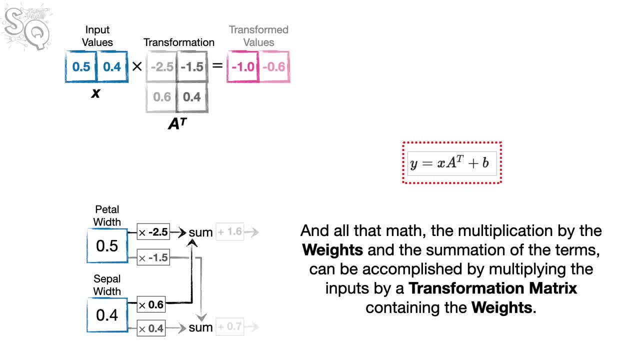 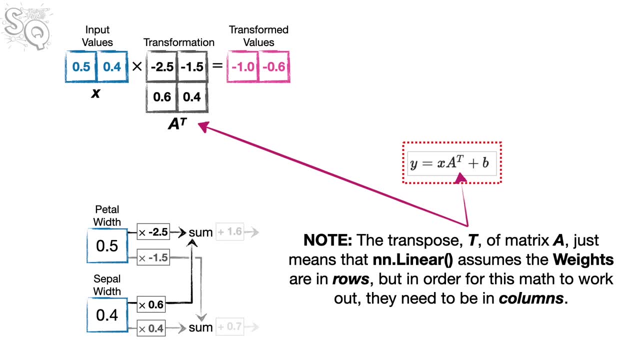 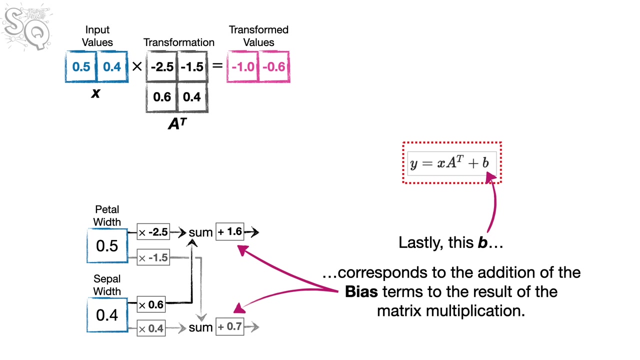 Note: the transpose T of matrix A just means that NNLinear assumes the weights are in rows, but in order for this math to work out they need to be in columns. Lastly, this B corresponds to the addition of the bias terms to the result of the matrix. 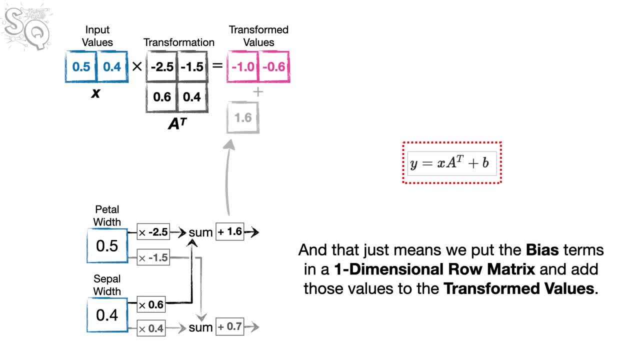 multiplication, And that just means that we put the bias terms in a one-dimensional row. So we just put the values in a one-dimensional row matrix and add those values to the transformed values. Thus this simple neural network multiplies and adds these matrices, and that corresponds. 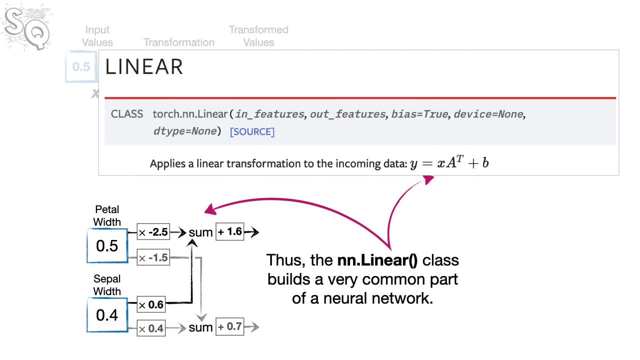 to this matrix equation. Thus the NNLinear class builds a very common part of a neural network. And do you remember how early on in this StatQuest we made a big deal about linear versus non-linear transformations And how a linear transformation means a constant change in the input, results in a constant? 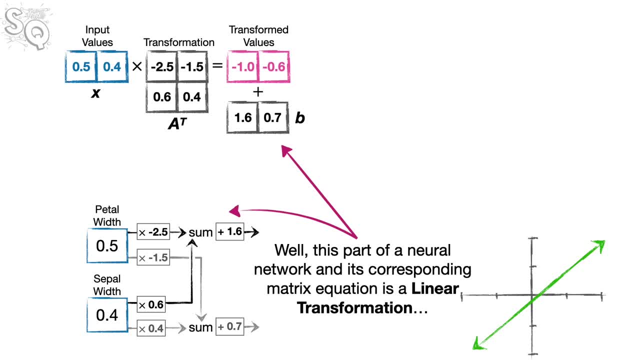 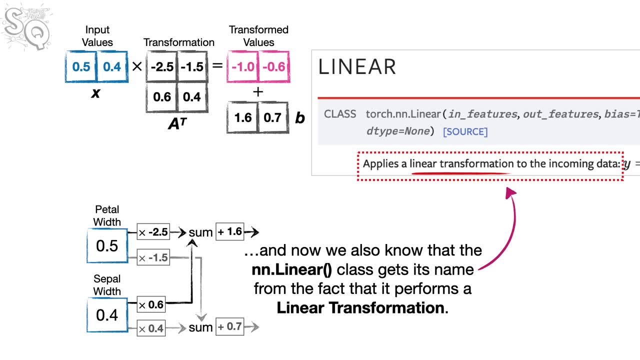 change in the output. Well, this part of a neural network and its corresponding matrix equation is a linear transformation. And now we also know that the NNLinear class gets its name from the fact that it performs a linear transformation. Now let's talk about this error message. 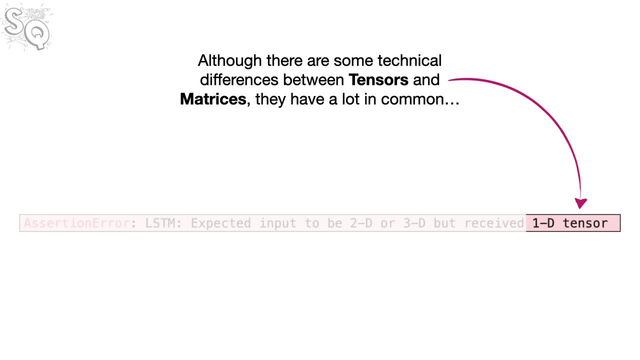 Although there are some technical differences between 10th and 15th. there are some technical differences between 10th and 15th, Although there are some technical differences between 10th and 15th. However, we know that tensors and matrices have a lot in common. 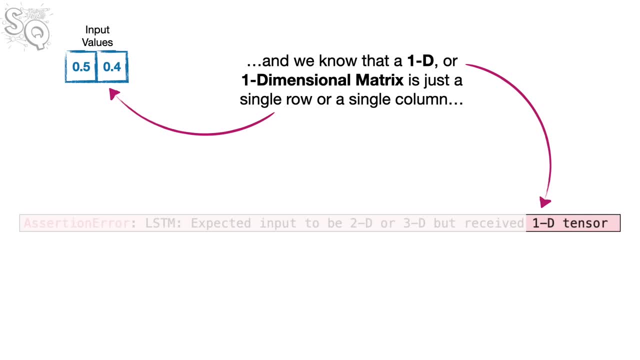 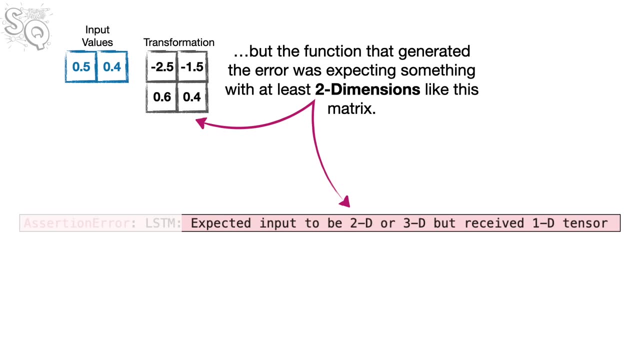 And we know that a 1D or one-dimensional matrix is just a single row or a single column, But the function that generated the error was expecting something with at least two dimensions, like this matrix. So the error just means we need to think a little bit more about the data we are giving. 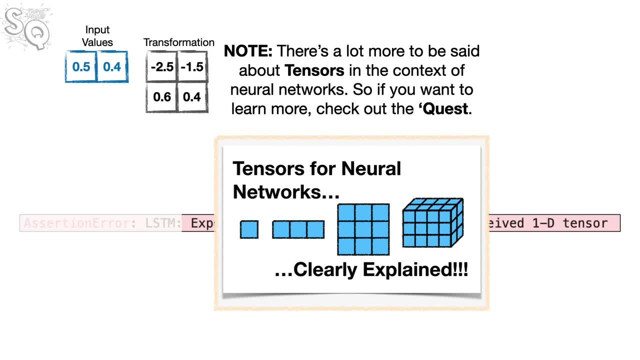 the function. There's a lot more to be said about tensors in the context of neural networks. So if you want to know more about tensors, go to the NNLinear classcom to learn more. check out the quest. Lastly, this is the equation for attention which is used by: 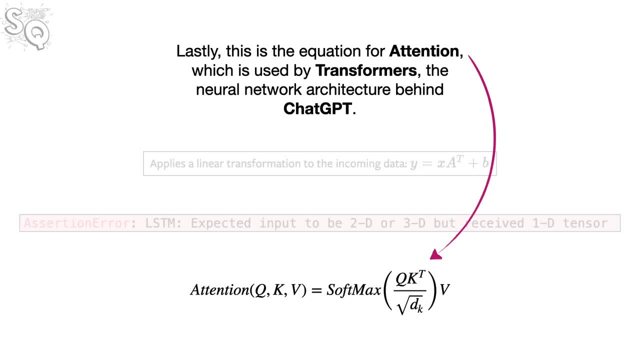 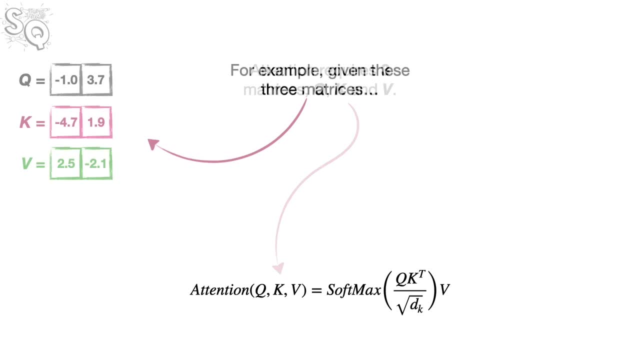 transformers, the neural network architecture behind ChatGPT. Attention requires three matrices: Q, K and V. For example, given these three matrices, the first thing we do is multiply Q by the transpose of K And given these example matrices, that gives us 11.7.. 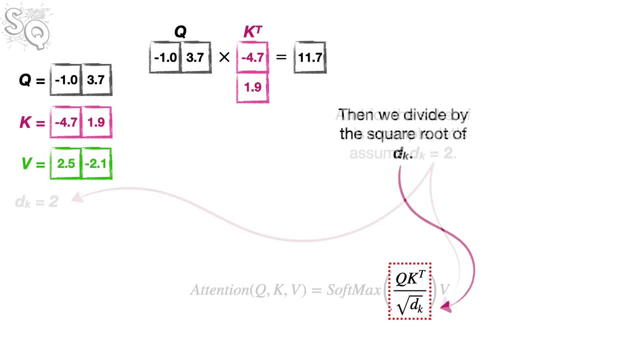 Then we divide by the square root of d sub k, And for the sake of this example let's assume d sub k equals 2.. So we divide 11.7 by the square root of 2, and that gives us 8.3.. 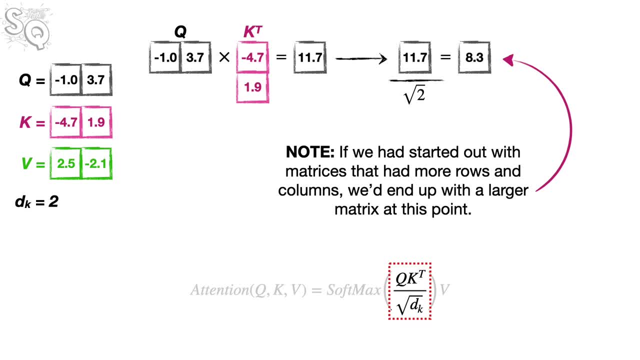 Note, if we had started out with matrices that had more rows and columns, we'd end up with 11.7.. larger matrix. at this point, And to be clear, attention is expecting larger matrices and that is why these variable names are capitalized. However, we're just using row matrices because